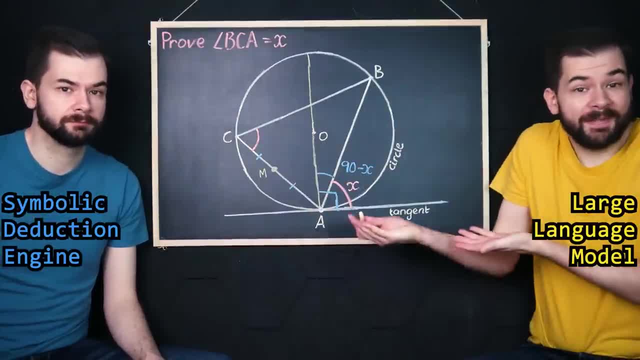 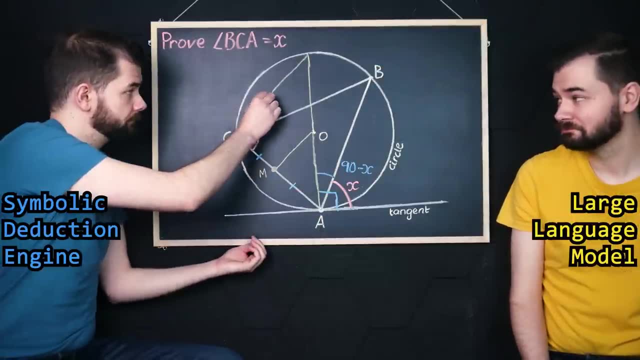 work in tandem, with the first making a suggestion- let's draw these lines- and the second making deductions, Because M and O are midpoints, these lines are parallel and they repeat until they reach the midpoint of AC. therefore, AM equals CM. The second is a symbolic deduction engine. I suggest ideas like plot: the midpoint of AC, therefore this is a right angle. and the third, making deductions. These two systems work in tandem with the first, making deductions, Because M and O are midpoints, these lines are parallel and they repeat until the 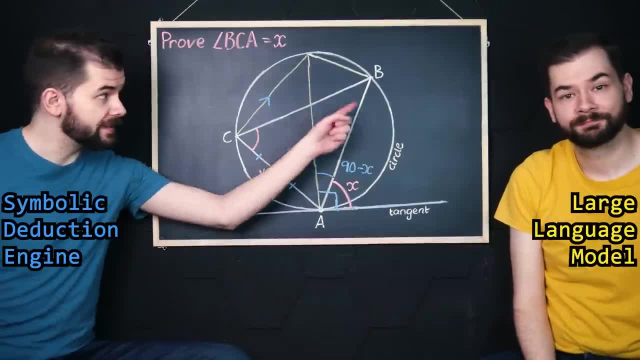 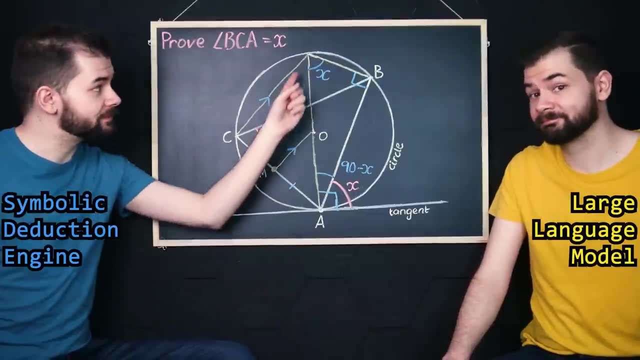 problem is solved. Now let's draw this line. By Thales's theorem, this is 90.. Angles in a triangle sum to 180, so this must be X, And by angles in the same segment, this is also X. 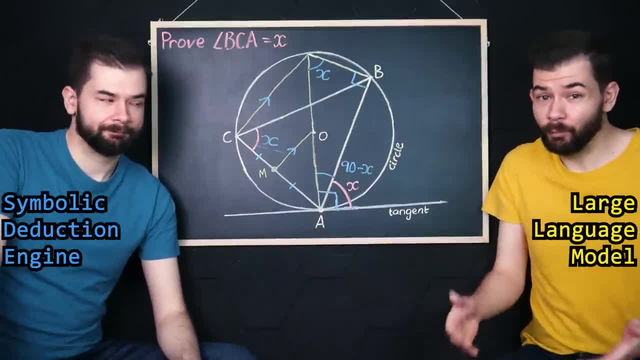 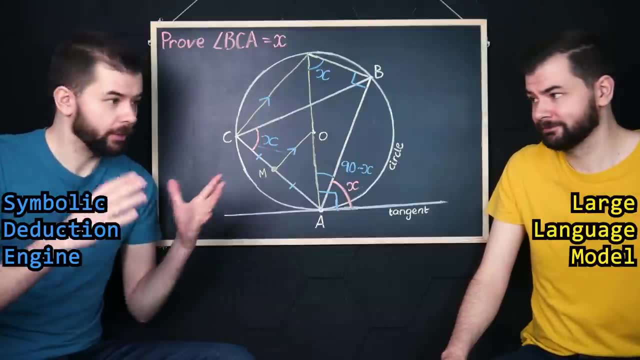 Well done, guys. I don't always have the best ideas, but we usually get there. I'm always right, but my options are limited by this absolute moron who doesn't know what's right. Some commentators have likened this to a right brain generating ideas and a left brain. 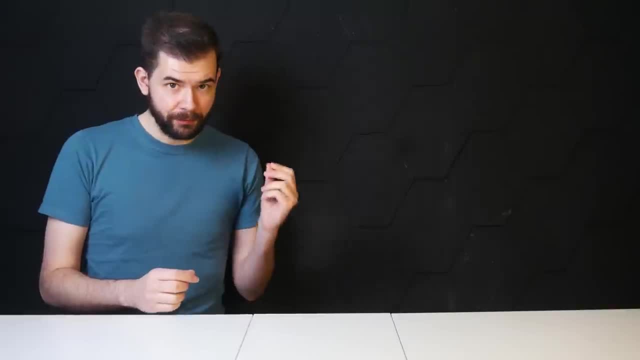 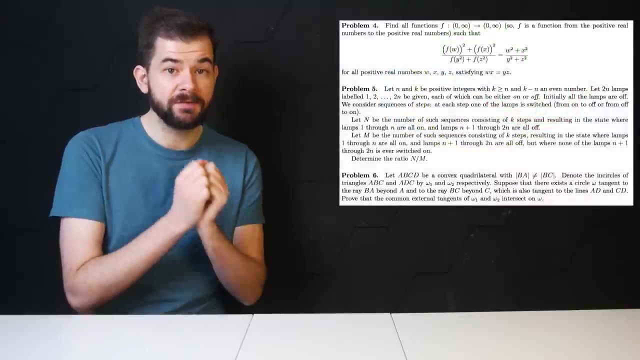 analysing the facts, Let's see it in action with a more challenging problem. The International Mathematical Olympiad is one of the world's toughest mathematics papers for high school students, with each paper containing six problems selected from four mathematical domains. Let's focus on problem one of 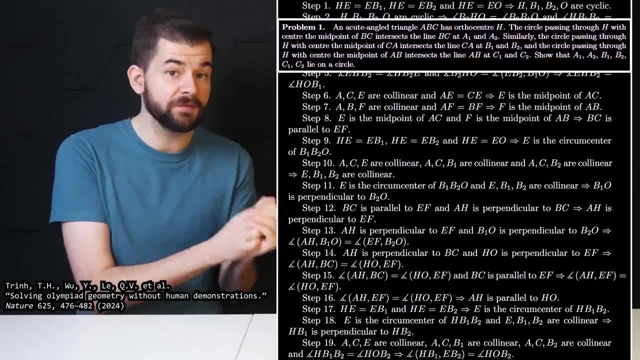 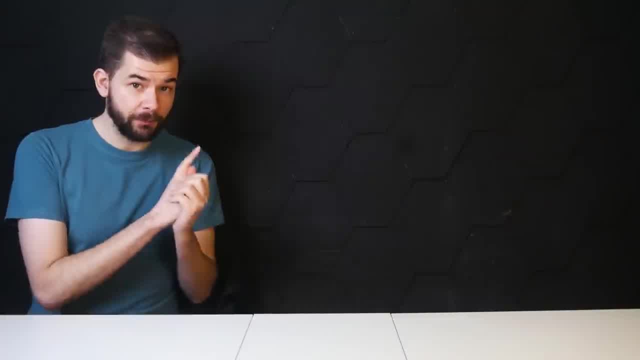 the 2008 paper, since alpha geometry solved this in 40 steps, which is fairly close to its average of around 55 steps. Before we state the problem, there might be some language with which you're unfamiliar, So here's a quick rundown of 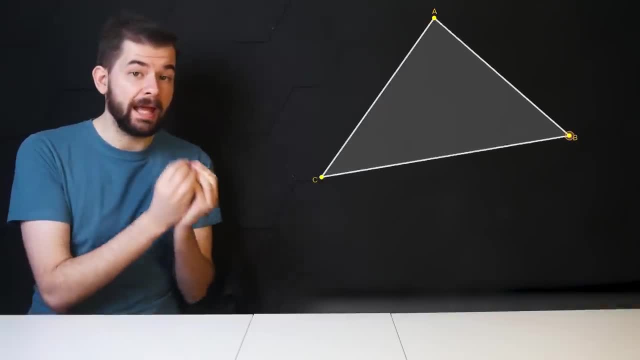 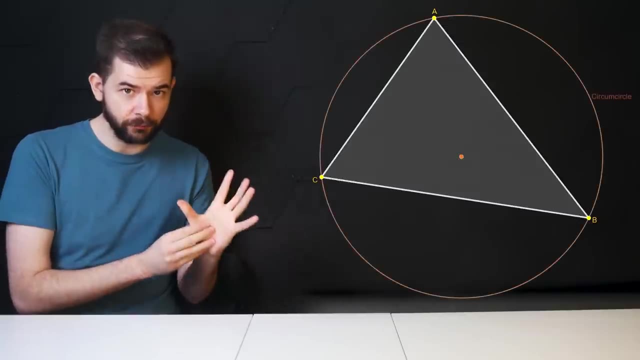 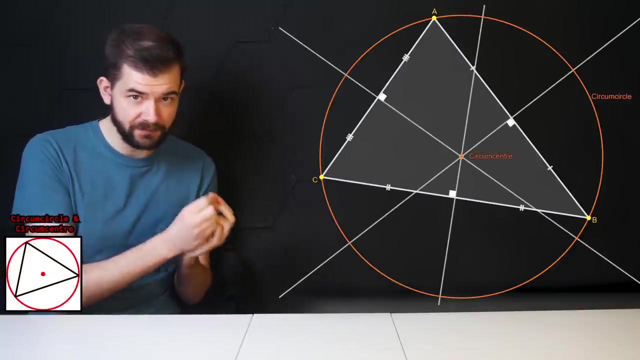 some triangle properties Start with a triangle ABC, and first it turns out that it can be embedded in a unique circle called the circumcircle, and its center is called the circumcenter. The center is the intersection of the perpendicular bisectors of the three edges, and I'll leave it as an exercise to justify why. 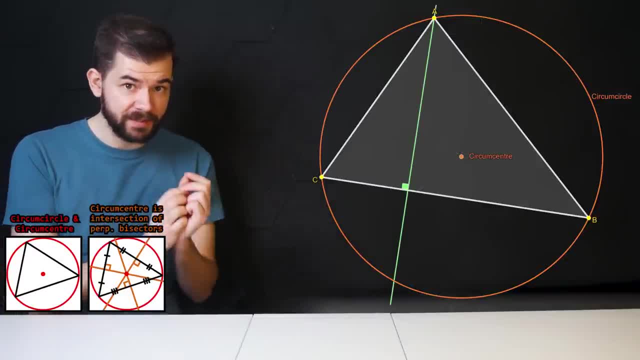 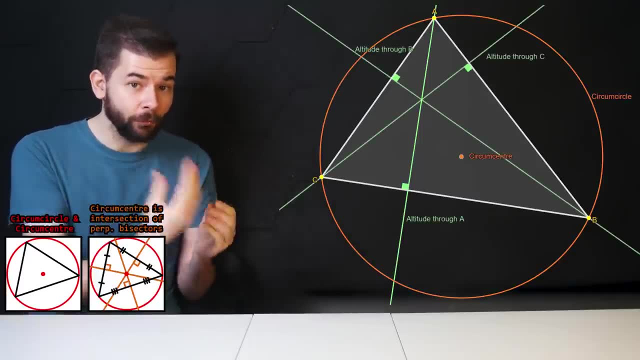 Second, a line from a vertex meeting the opposite edge at a right angle is called a hexagon. Now the hexagon is a line from a vertex meeting the opposite edge at a right angle is called a hexagon. Third, an altitude. Every triangle has three. and third, it turns out that all three altitudes meet at a common point called the orthocenter. 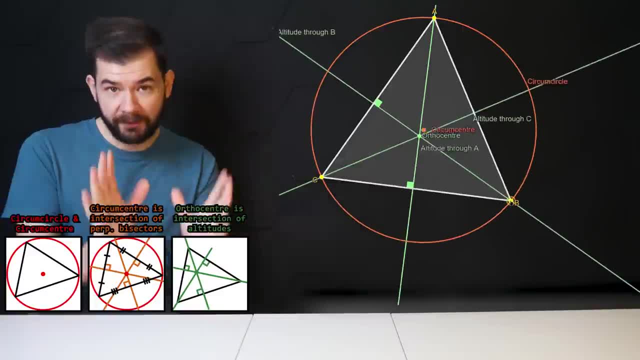 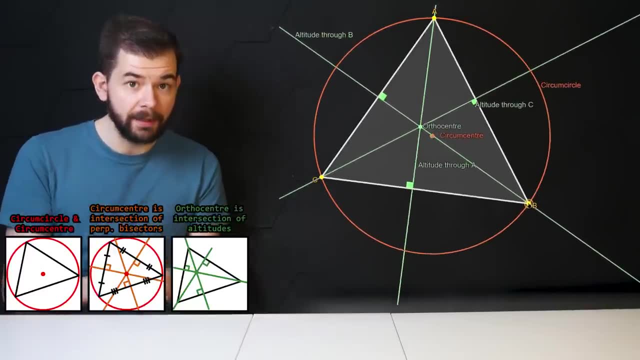 Ortho, meaning orthogonal, meaning perpendicular, meaning at right angles. you get the idea. Pause here. if you need to just digest this, I'll summarize them here as I'll be using them for the rest of the video. The extended cut of this video goes into a bit more detail on these, like why the circumcircle and 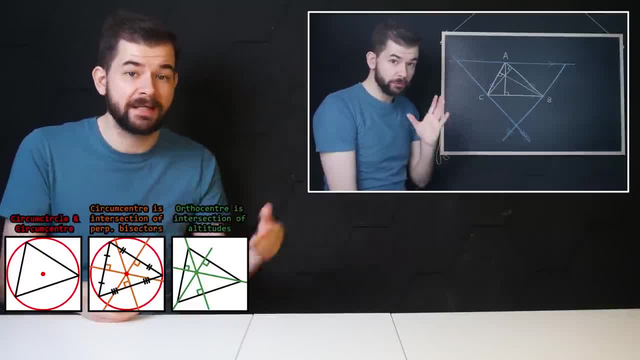 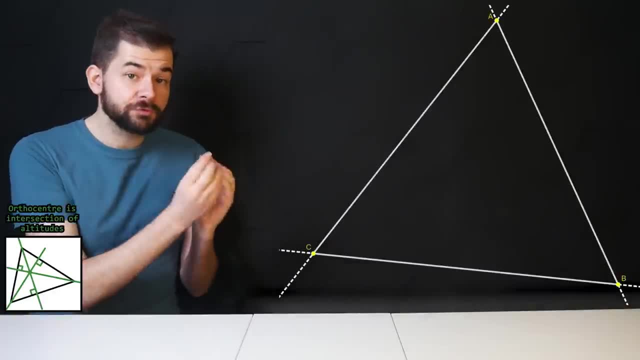 orthocenter even exist, and if you want to check that out, as well as extended cuts of other videos, please consider supporting me on Patreon. So let's now look at this Olympiad problem. We'll start with some triangle ABC and plot its orthocenter H. 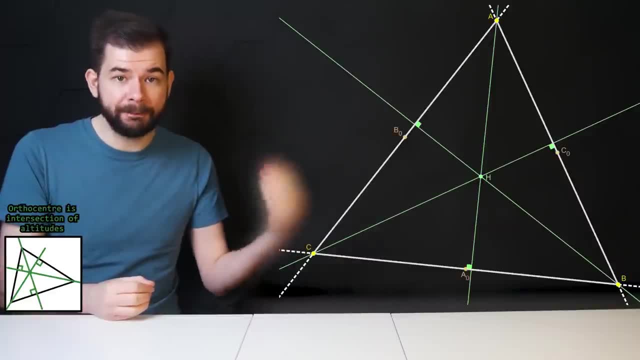 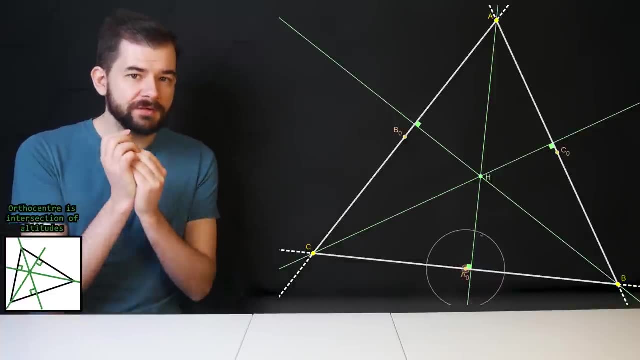 Take the midpoints of the three edges and label them A0, B0, C0,, so that A0 is opposite A, B0 is opposite B, C0 is opposite C. Now draw a circle centered at A0, which goes through H. 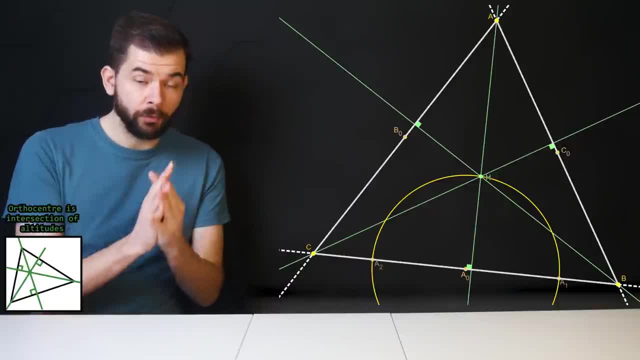 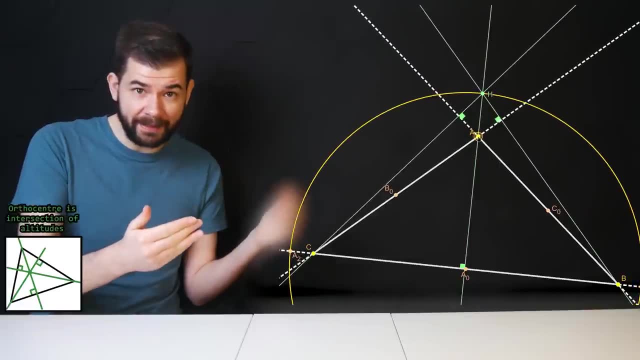 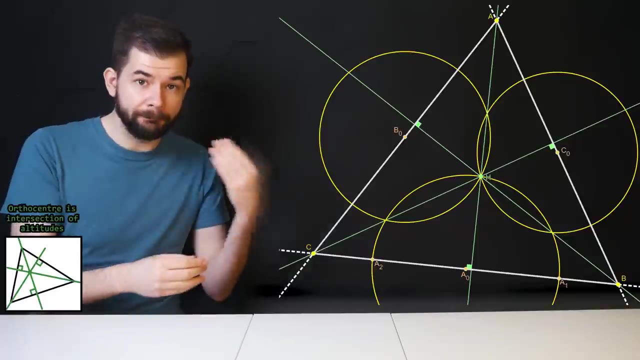 Now this circle will cross BC twice. Call these points A1 and A2.. These needn't actually be on the triangle- In an obtuse triangle they might drift outside, but we plot them anyway. Now draw circles centered at B0 and C0, each crossing H, and plot B1 and B2, C1 and C2 in the same fashion as A1 and A2.. 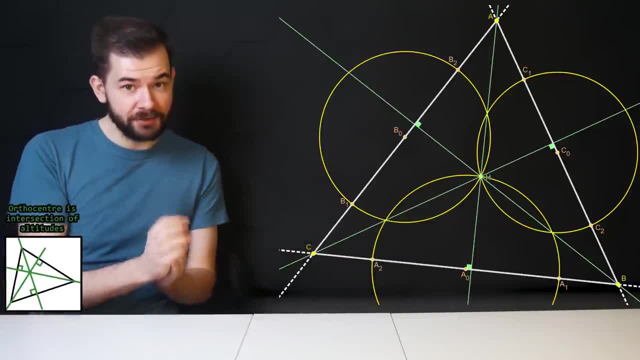 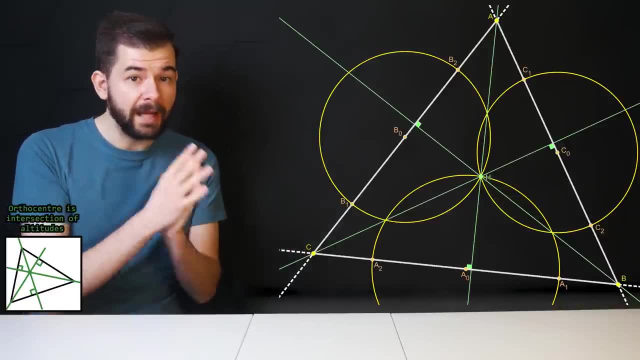 These problems really tend to front-load a lot of information. so pause and digest this if you need to, because now here's the question. We want to prove that A1, A2, B1, B2, C1 and C2,. 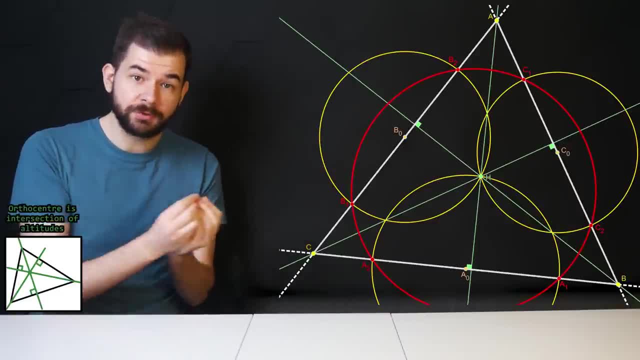 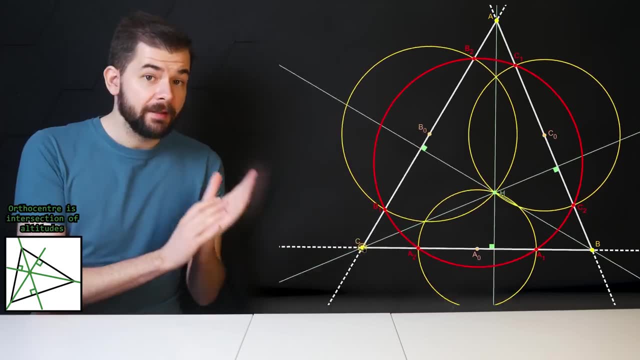 all lie on a circle. In Geogebra we can see that this seems to be true, But our task is to prove it. Pause now, if you want to have a crack at it. then we'll look at alpha geometry's solution. 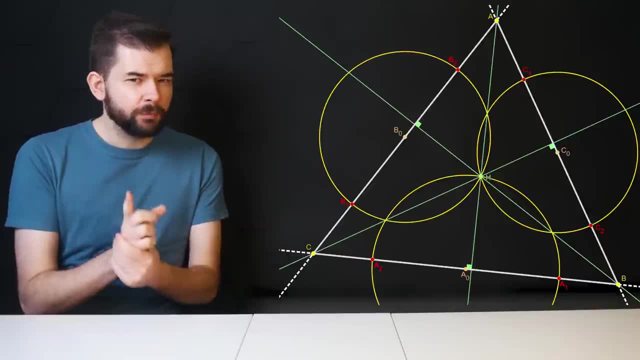 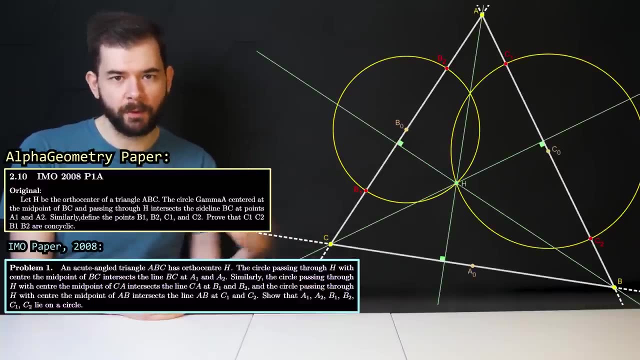 So how did alpha geometry solve this problem? Well, first, it's worth noting that in the paper on alpha geometry the problem is stated differently. just wanting to prove that B1, B2, C1 and C2 are cyclic. This is insufficient. By symmetry, a proof of this kind. 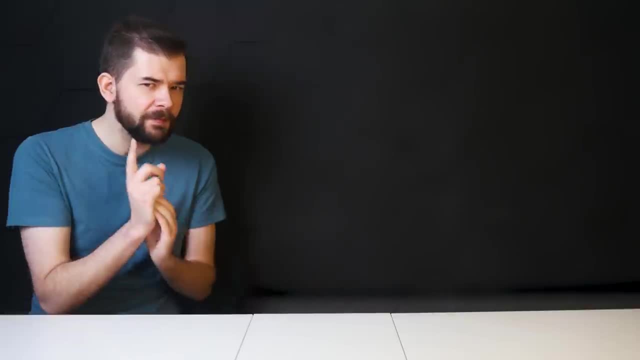 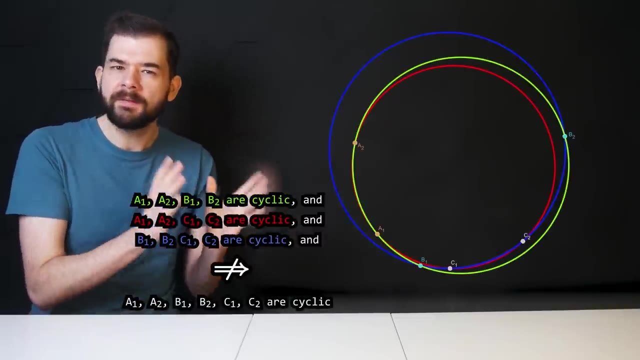 will generalize to the other pairs of sides, but it could be the case that the A's and B's, the A's and C's and the B's and C's share different circles. But anyway, maybe they'll justify why this is sufficient later. Just a few things to mention up front. There are often a few. 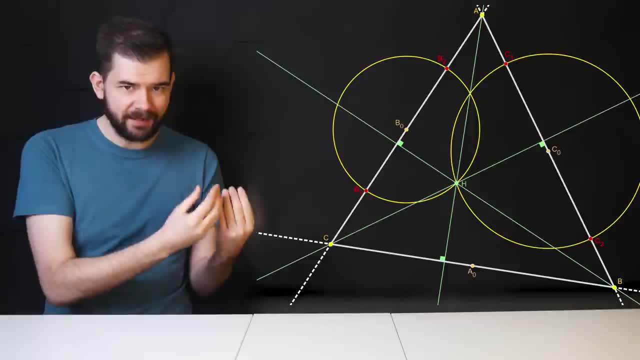 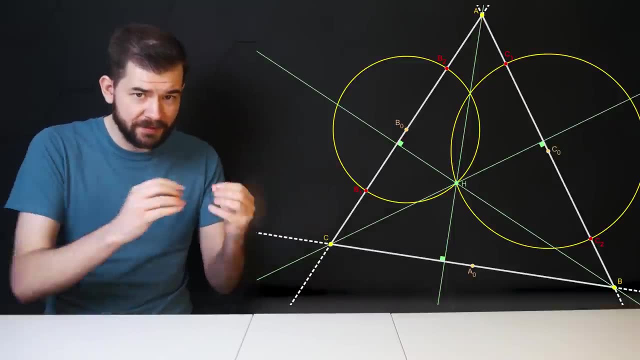 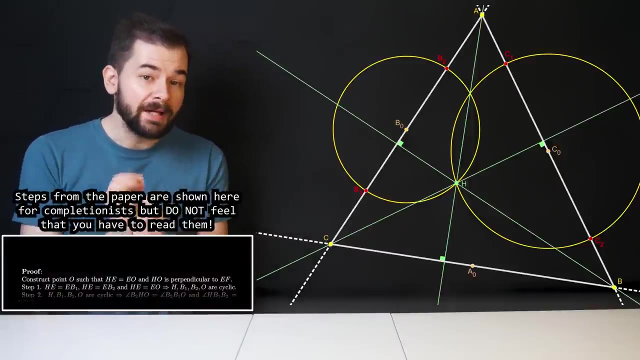 redundant steps along the way. It often restates things already deduced. This is due to how it presents solutions, but I'll mostly just gloss over them and sometimes compress steps together. But I will show all steps on screen. if you care about the minutia, I'll assume a high school. 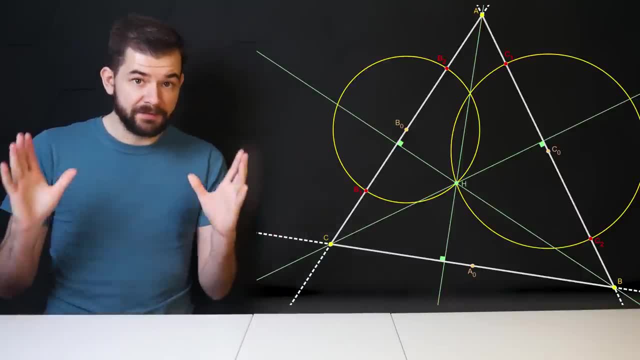 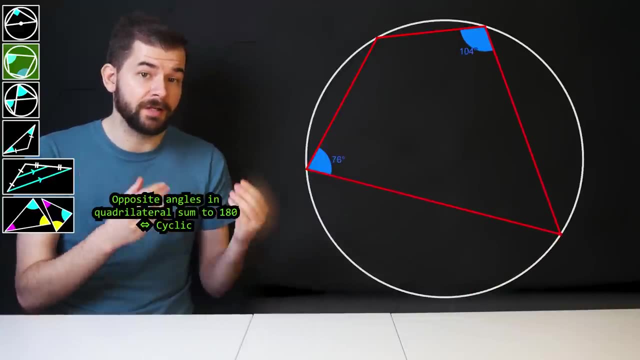 knowledge of geometry throughout. The results we'll need will be summarized here. One to draw your attention to is cyclic quadrilaterals. Most of us learn that opposite angles in a cyclic quadrilateral sum to 180, but the converse is also true If you have a quadrilateral where opposite 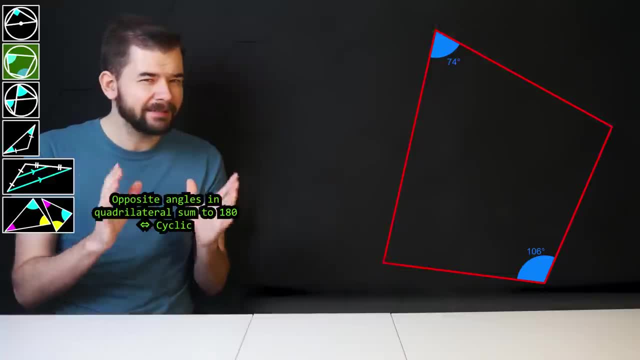 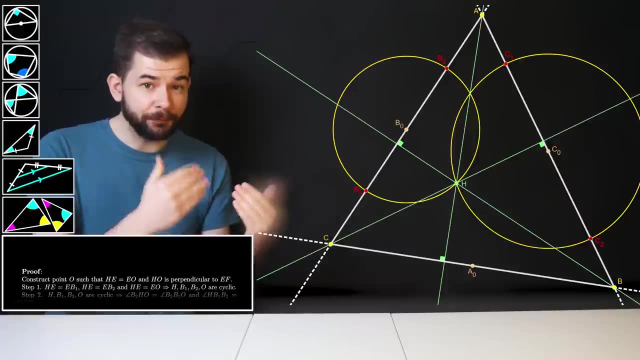 angles sum to 180, then it is cyclic. That's less obvious and it's going to be very important. I will show all steps on screen. if you care about the minutia, I'll assume a high school knowledge will be going through the steps fairly quickly. Each step is fairly simple, but the length of the 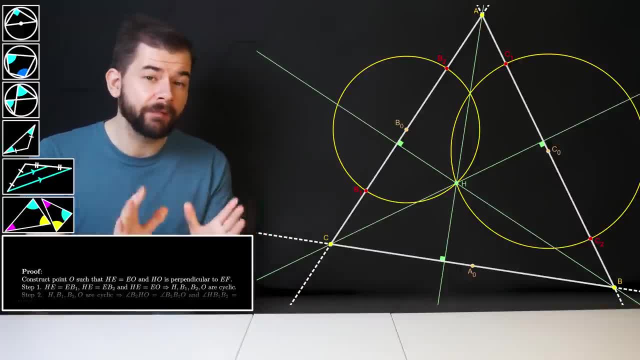 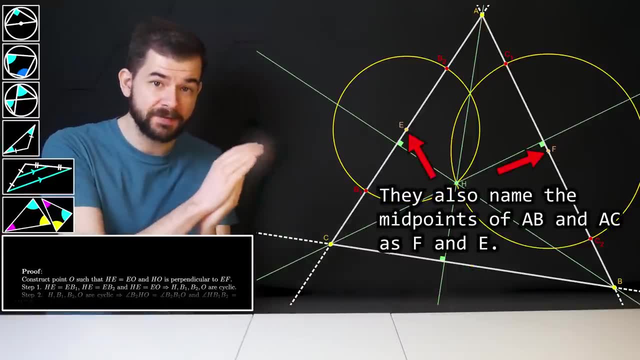 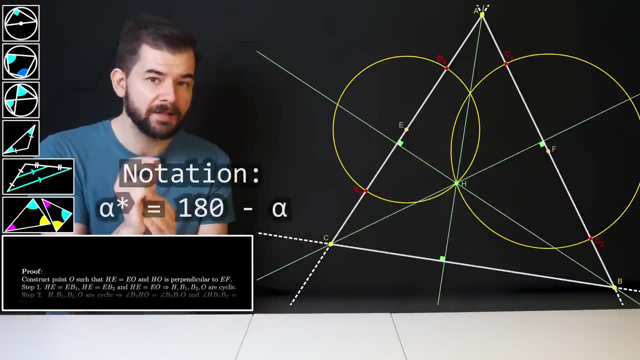 proof is quite overwhelming. My advice is not to worry about every little detail and just get a feel for alpha geometry's approach, but feel free to pause after every step if you want to fully grasp every detail. I'll use lowercase Greek letters for angles and I'll use a star to denote. 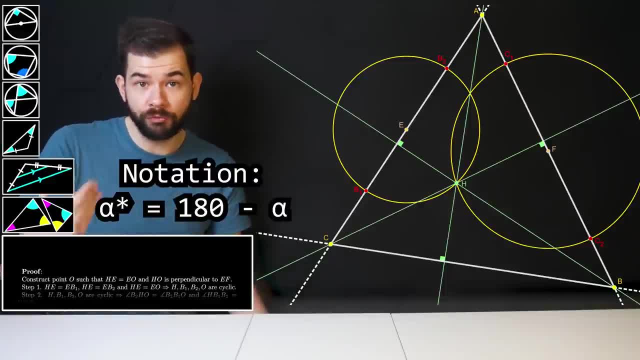 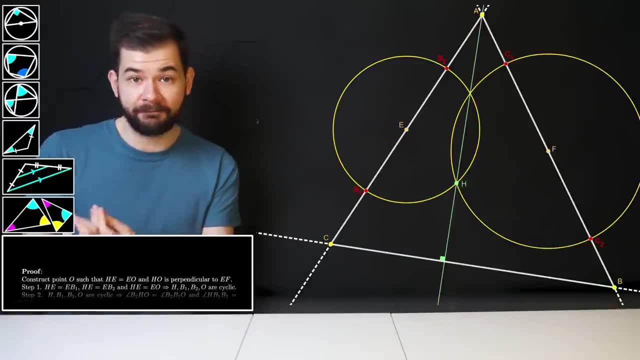 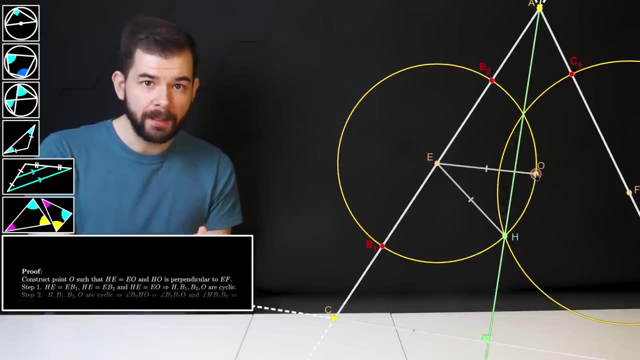 a supplementary angle. ie alpha star is 180 subtract alpha. Let's get into it. We actually don't need these altitudes, so I'll hide them. and it starts by defining point O such that EH equals EO, So clearly O must lie on this left circle, but also such that HO is. 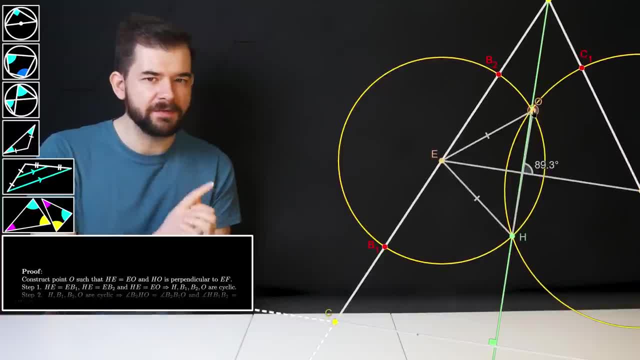 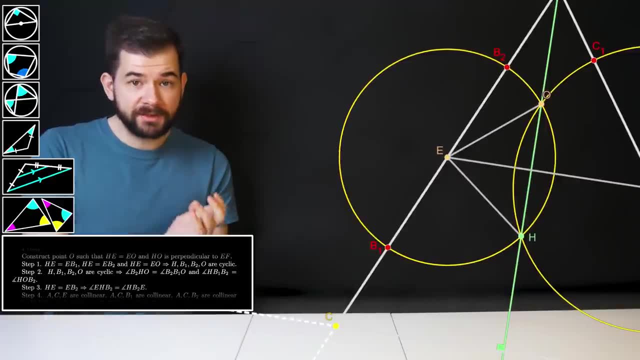 perpendicular to EF, I think we can infer that O is actually where these circles intersect. but alpha geometry doesn't realize this yet. Step one is realizing that O must lie on the left-hand circle, so that's good. And step two: it uses angles in the same segment. 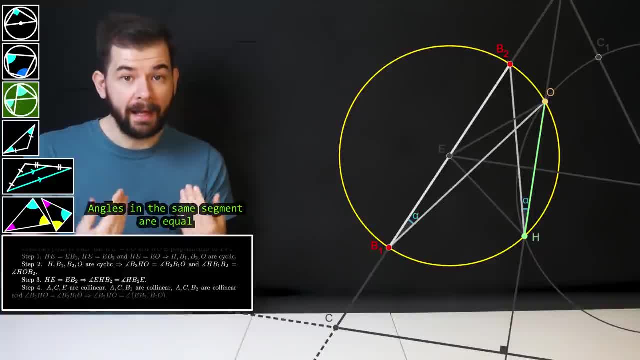 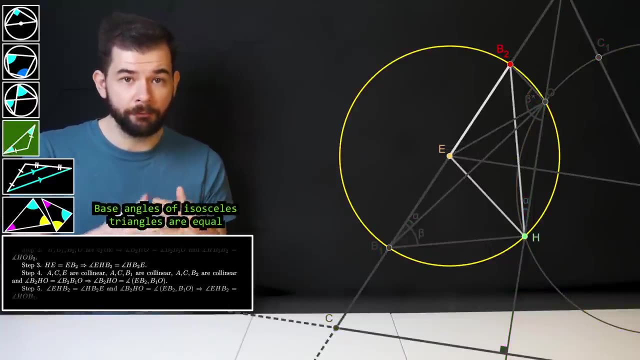 to prove that these are the same, I'll call them alpha. Also, this is a cyclic quadrilateral, so these angles are supplementary. They sum to 180.. I'll call them beta and beta star. Step three: this triangle is isosceles, as EB2 and EH are both radii of this circle. 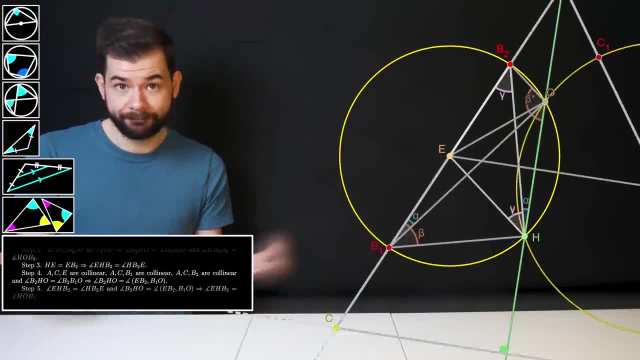 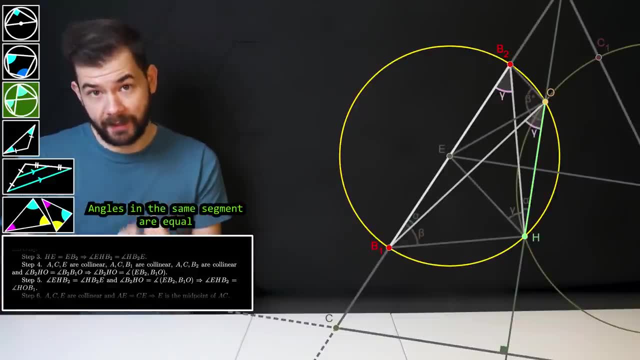 so these angles are the same and I'll call them gamma. Steps four and five: here it infers that this angle is also gamma. Again, this is by angles in the same segment. Steps six to eight: it deduces that EF is parallel to BC, by acknowledging that E and F are 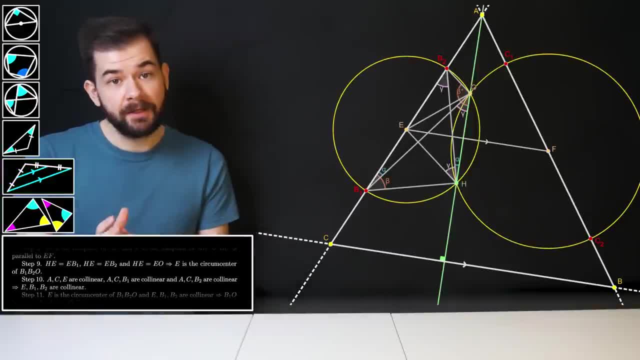 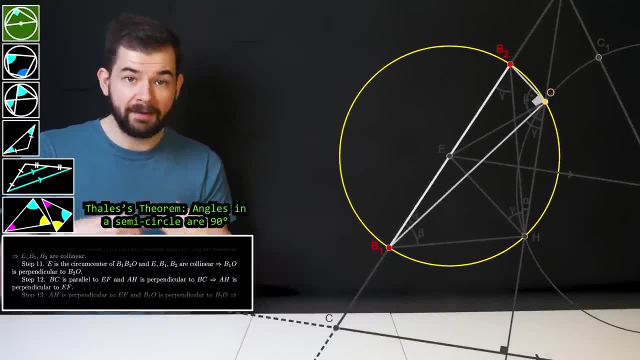 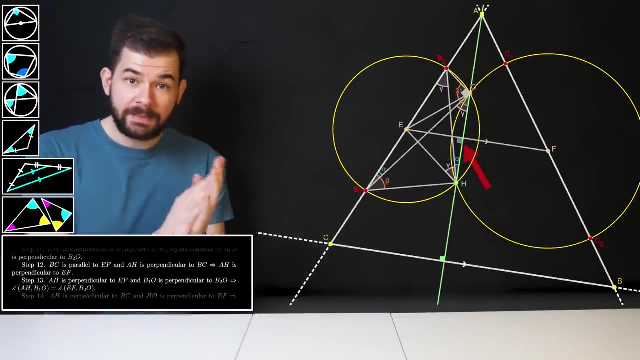 midpoints of those lines of the triangle. Steps nine and 10 are some of the redundant steps I mentioned earlier, And step 11, we have that this is a right angle and that's by Thales' theorem: Angles in a semicircle are 90 degrees. Step 12, AH is perpendicular to EF. That's because AH and BC. 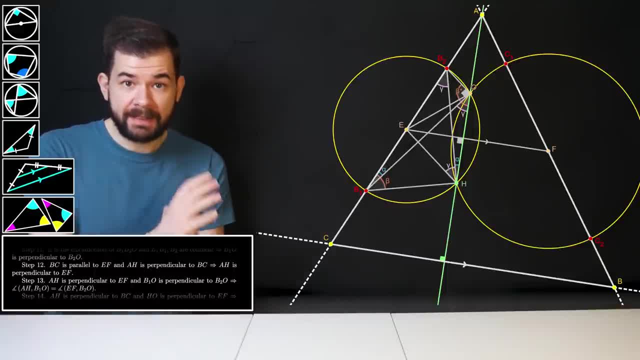 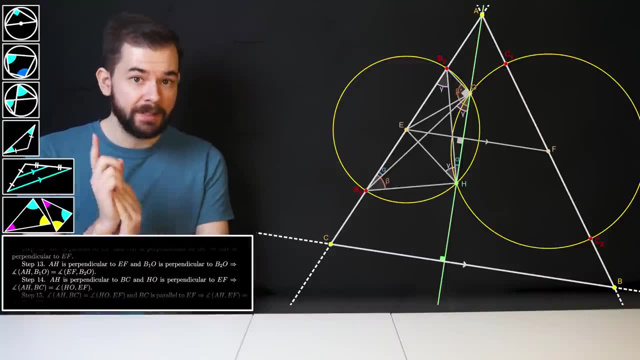 are perpendicular by the definition of an altitude. BC and EF are perpendicular to EF, Steps 13,. now this one is interesting. We extend the line B2O to EF. I guess that's the right brain talking. We've run out of angles to chase, so let's just stick another line in. 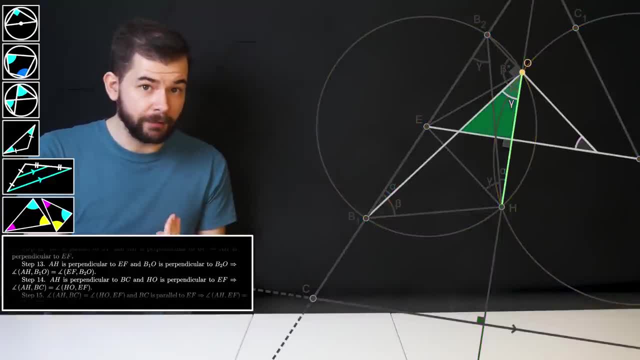 Now, what's this angle here? Well, we have a right angled triangle, so this is 90 subtract gamma. but here is another right angled triangle, so this angle must be 90 subtract, 90 subtract gamma. In other words, it's gamma. 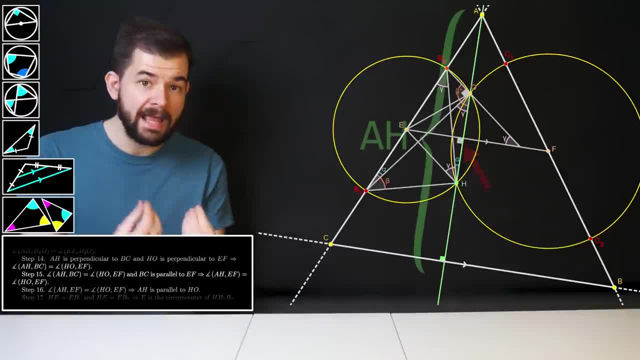 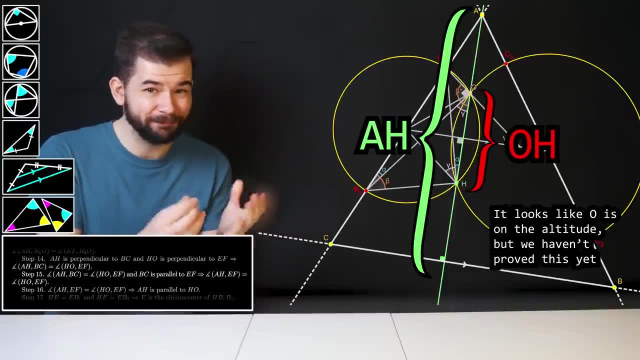 Steps 24, and then we get a right angle, and then we get a right angle. Now, after we've explained the right angle, we're going to go into the right angle. Now, when it comes to diagrams, I suggest I use this common right angle here. 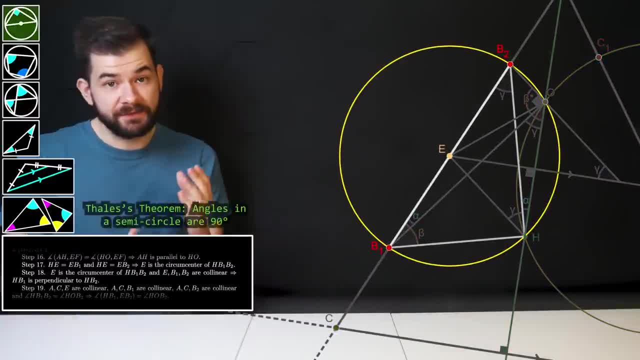 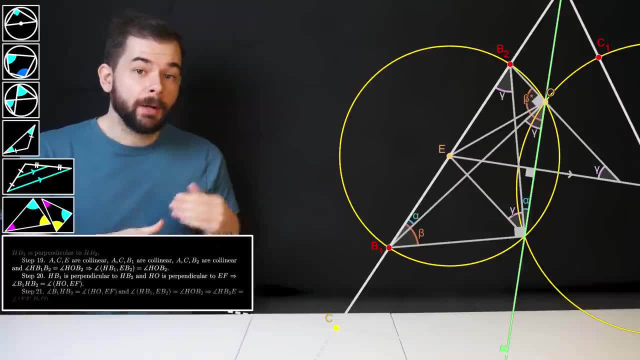 to establish that AH is parallel to OH. The diagram is awkward here because it looks like this is necessarily the case, and it is, but alpha geometry didn't know that yet. Steps 17 and 18, this is a right angle, And again that's by Thales' theorem. Steps 19 to 22 are more redundant restatements And Step 23,. this is an isosceles triangle as EB2 and EO are radii, So these basic equations are the same pattern. So a right angle there, right angle there, And this is a right angle. 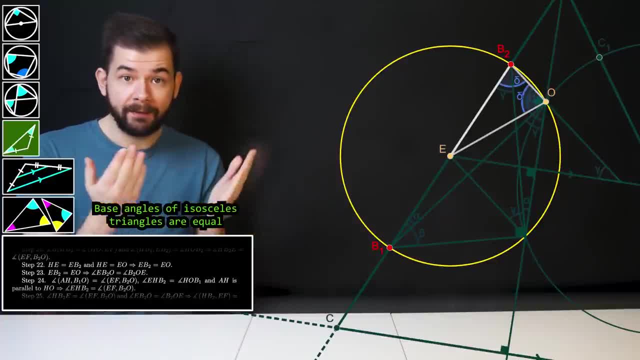 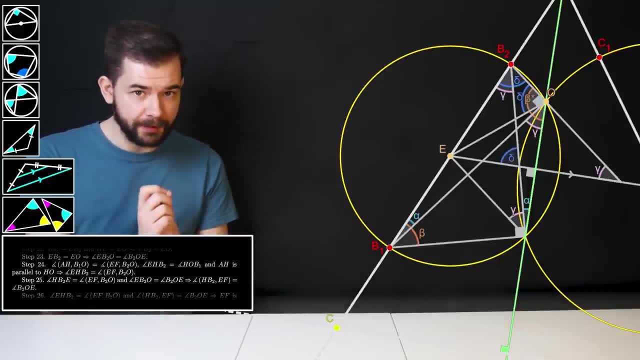 So again, that's by Thales' theorem, Or this is a right angle. angles are the same, and I'll call them delta, Steps 24 and 25. now, this is a brilliant inference, and that's that this angle is also delta. All it says as justification is that these are delta and 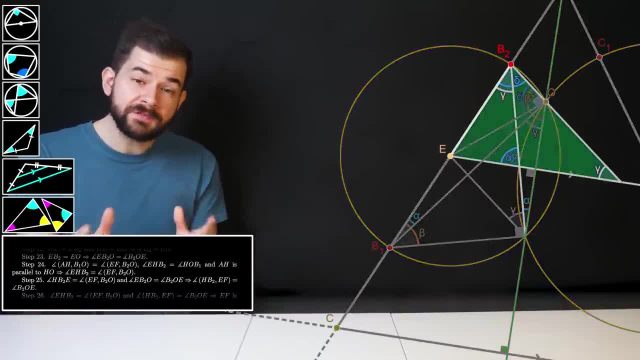 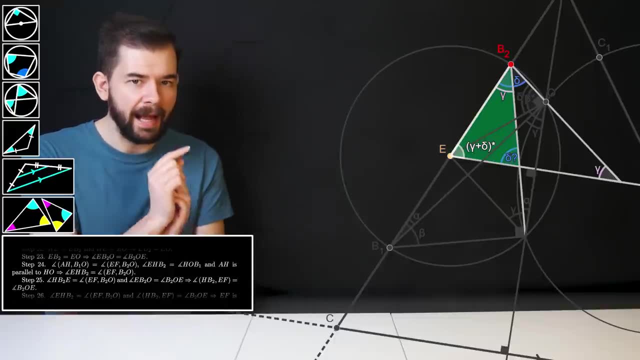 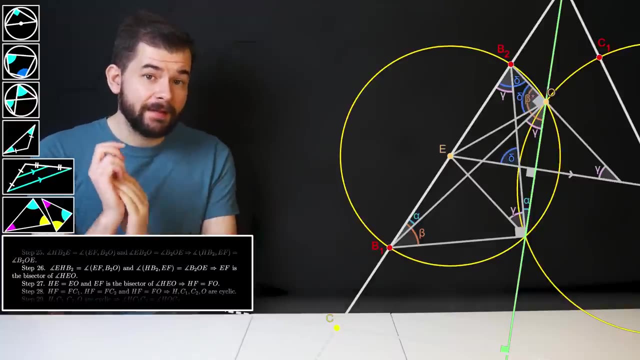 these are gamma, so why must this be delta? Well, here's a triangle with gamma and delta, so its third angle supplements them. but now here's a triangle with gamma and this angle, so its third angle must be delta, as required. Step 26: again, another fantastic inference, and that's that EF. 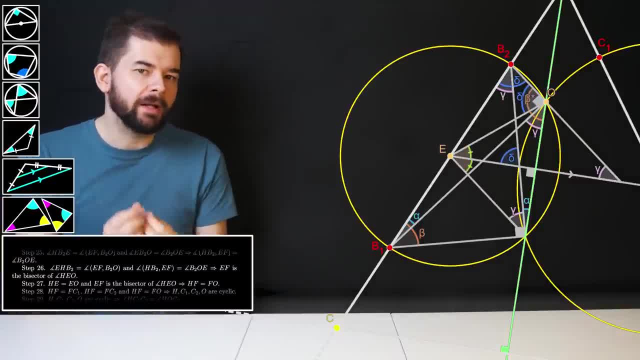 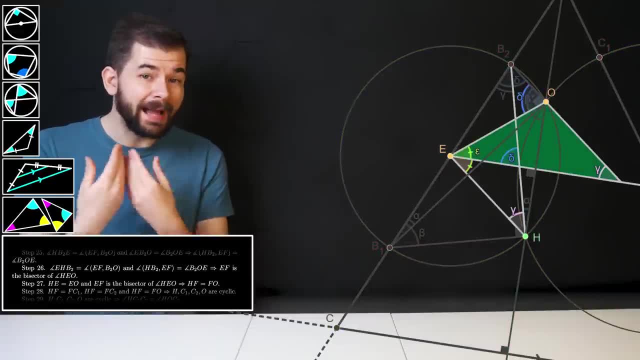 bisects this angle here. Now why is that? Well, call the top one epsilon, yes, that's how many of us pronounce it- and note this triangle up here whose top angle is delta star. So epsilon supplements gamma and delta star. and now note this triangle also with gamma and delta star. so this angle. 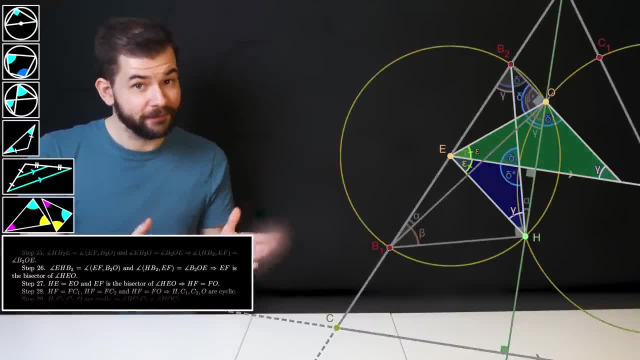 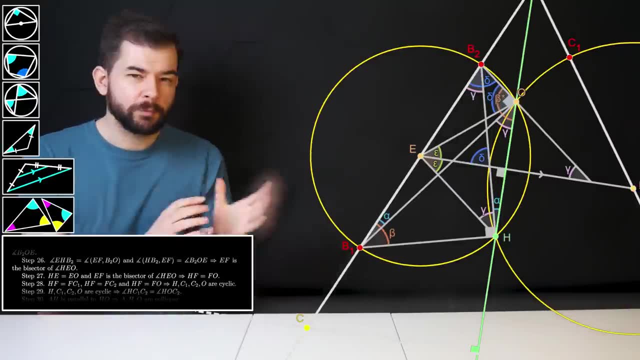 must be epsilon as well. It's great stuff. I mean, we can infer this so much more easily. but it is kind of cute how alpha geometry picks the most difficult ways to get there. Step 27, because F lies on the angle bisector of EO and EH, and 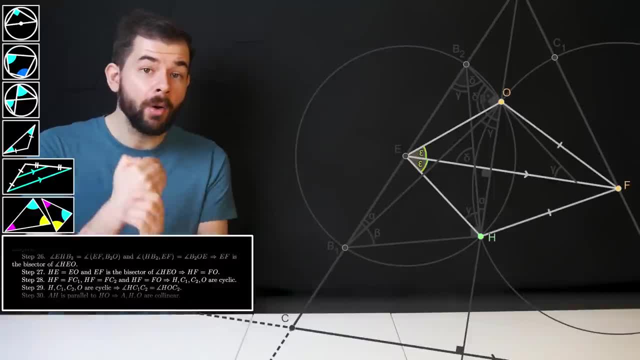 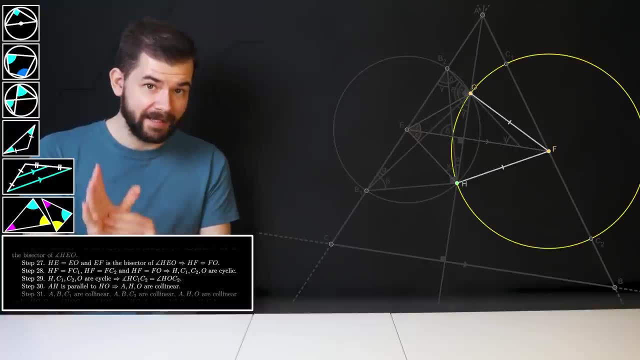 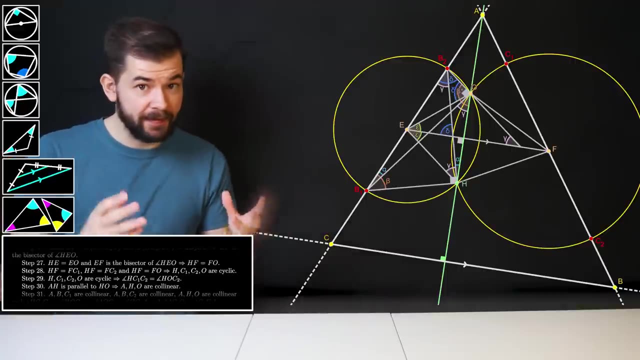 because EO and EH are the same length. we have that FO and FH are also the same length And step 28, therefore O, lies on this right hand circle. Remember when we said as much at the very beginning? I told you we'd get there eventually. Okay, so it's putting a lot of pieces together. 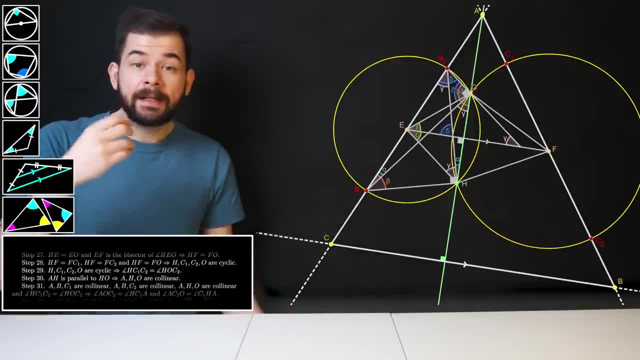 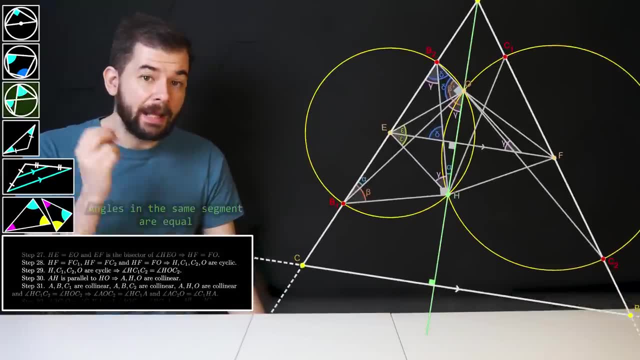 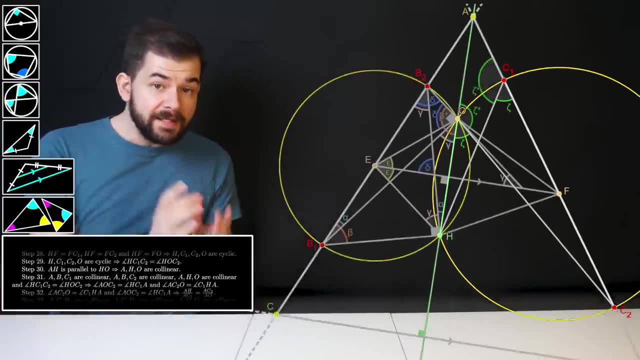 and step 29. what does it do with this newfound power? Well, what do you think? It's straight back to chasing the angles. So plot C2O and HC1.. Now these are the same via angles in the same segment and I'll call them zeta Steps 30 and 31. these are clearly the same as they're both zeta star and as 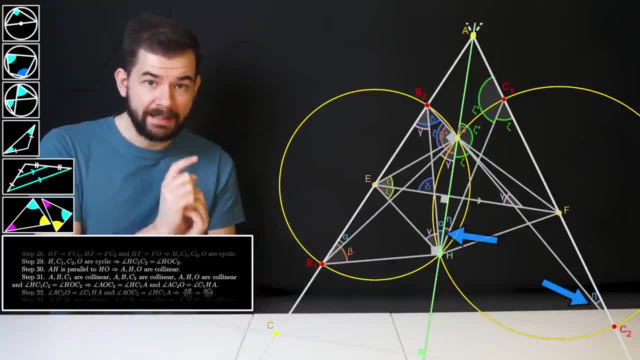 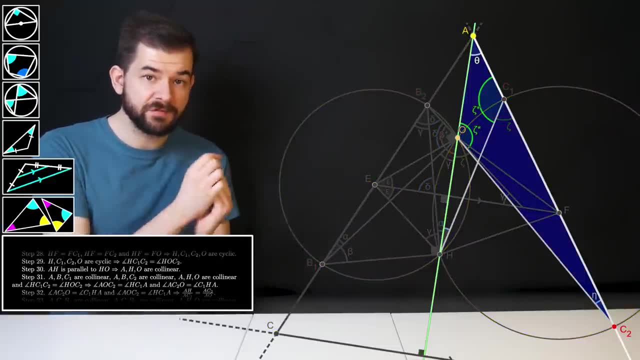 a result, these angles are the same. I'll call them eta. And why is that? Well, consider this triangle and call its top angle theta. Then eta supplements theta and zeta star. Now consider this triangle and we see that this angle also supplements theta and zeta star, so it must also be eta. Gonna need the whole Greek. 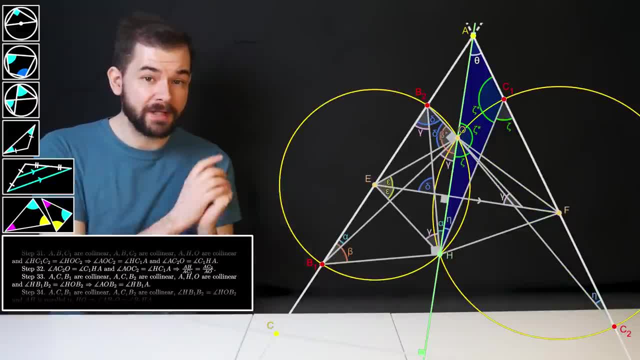 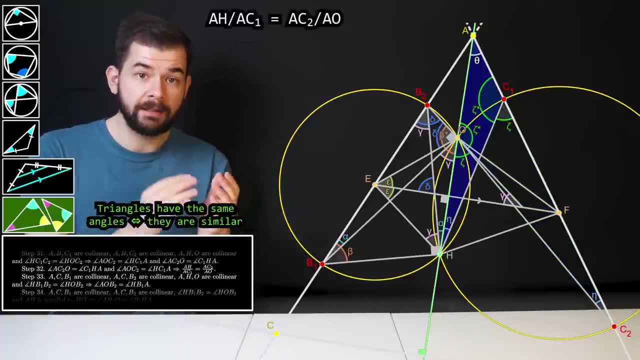 alphabet at this rate. Steps 32, because these triangles have the same angles, they are similar, and that's expressed as this ratio: AH over AC1 equals AC2 over AO. Steps 33 and 34: this is quite fiddly, but we're doing a similar thing on the left. 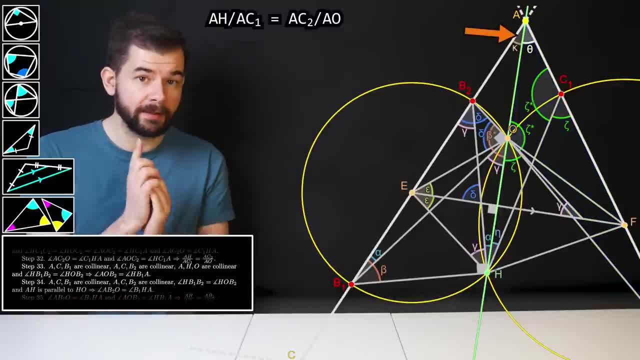 Steps 35 is the same as we did on the right with the zetas. So call this top angle kappa and fill in this angle which we know is beta. We'll need it in just a second. This angle is 90 plus alpha and we 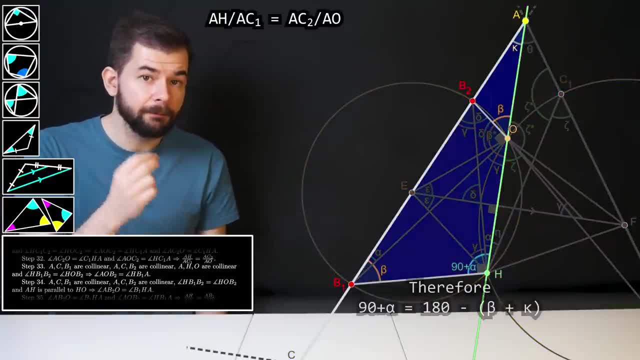 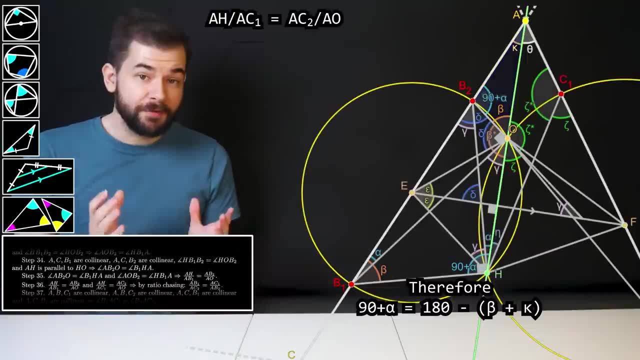 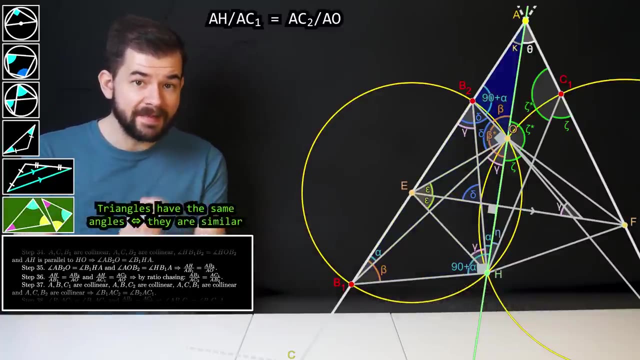 see that it is in a triangle with beta and kappa. But this angle is also in a triangle with beta and kappa, so it must also be 90 plus alpha Step 35, similar to before. no pun intended, these two triangles have the same angles, so they are similar and that's expressed as AH over AC2 over AC1. 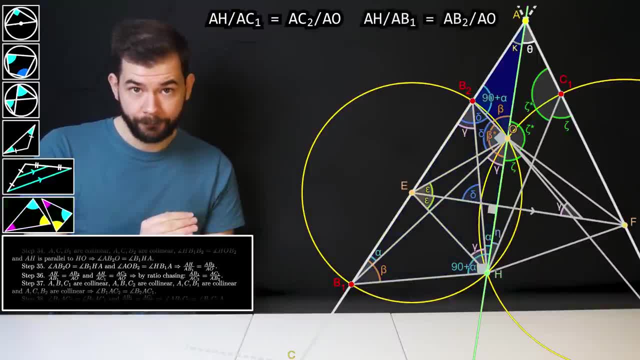 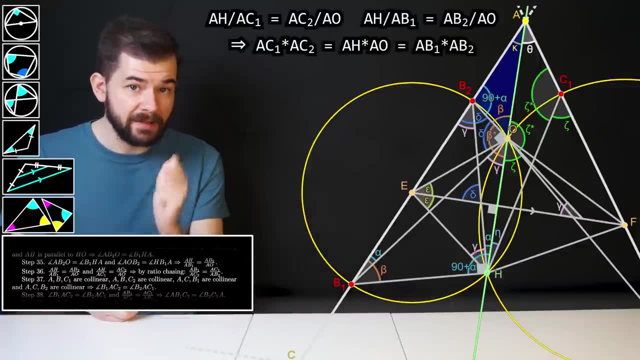 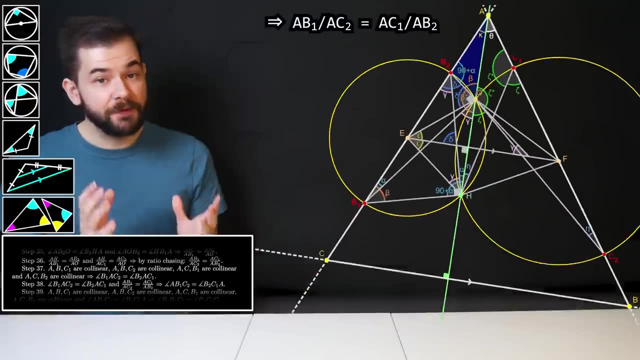 over AB1 equals AB2 over AO. Step 36, now a bit of algebra. we see that AH times AO is equal to AB1 times AB2 and AC1 times AC2.. Therefore, AB1 over AC2 is equal to AC1 over AB2.. Steps 37 and. 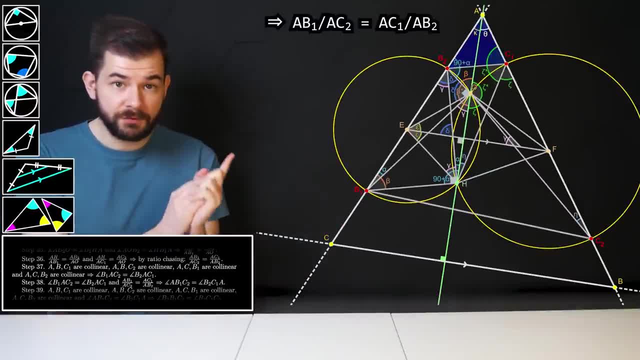 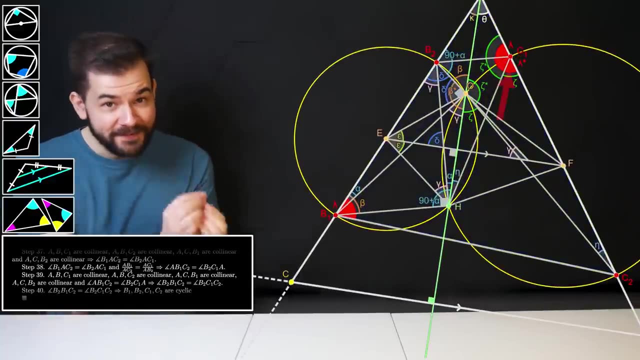 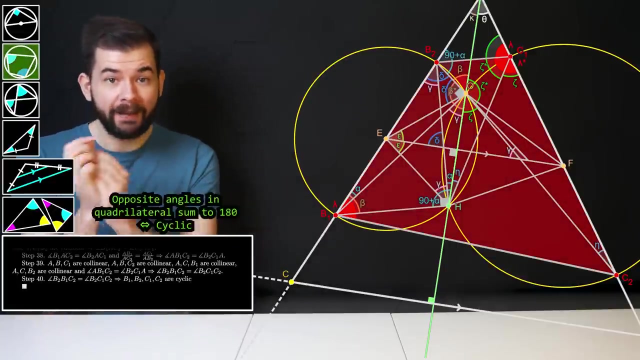 38,. we will use this ratio So construct B2C1 and B1C2, and this ratio tells us that these triangles are similar. thus their angles are the same, In particular these ones which I'll call lambda. Step 39,, so close, this angle supplements lambda, so I'll call it lambda star. And step 40,. finally, we have 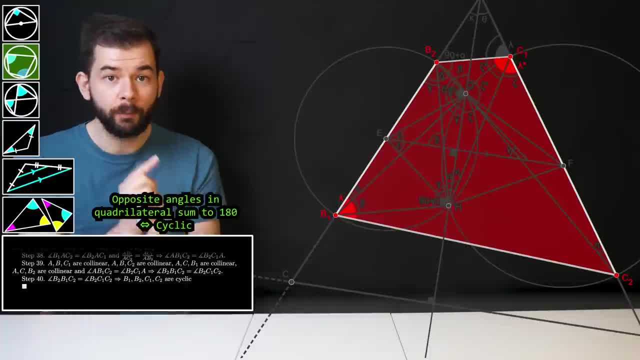 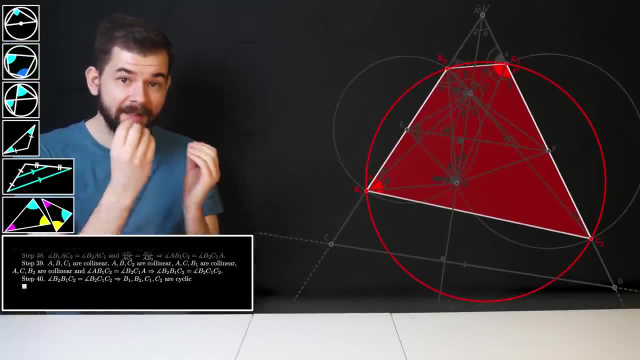 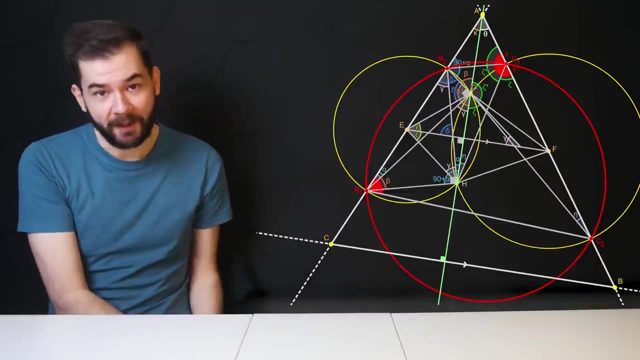 a quadrilateral, B1B2C1C2, with opposite supplementary angles. thus it is cyclic. Thus, these four points lie on a circle. Finally, so what do we think about this proof? Well, for a start, it doesn't really answer the question. 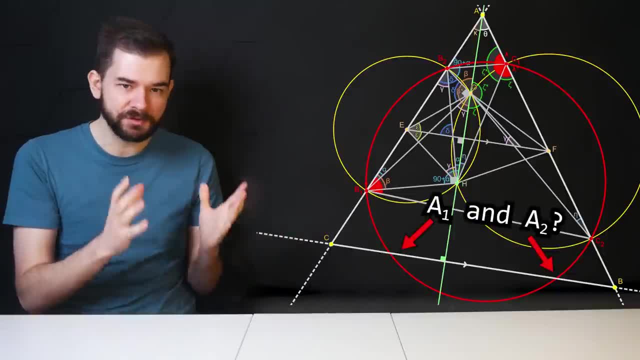 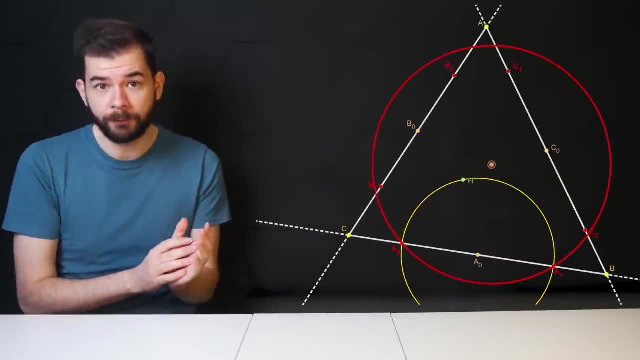 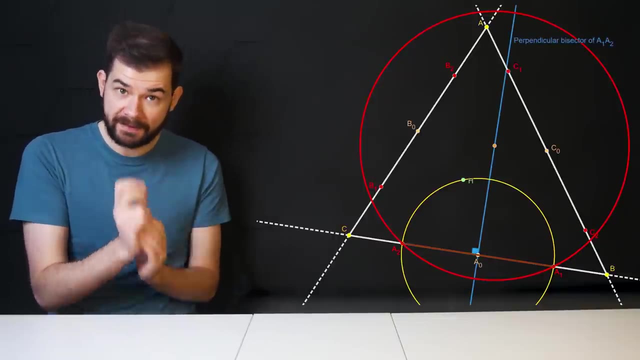 There is no demonstration that A1 and A2 must lie on this circle. Now, this is easy to argue, because consider any circle containing A1 and A2, then A1- A2 is a chord of the circle and its perpendicular bisector must contain the centre. But A1- A2 is a diameter of this circle centred at A0, therefore, A0 is a diameter of this circle centred at A0.. So if we consider any circle containing A1 and A2, then A1, A2 is a chord of the circle and its perpendicular bisector must contain the centre. But A1, A2 is a. 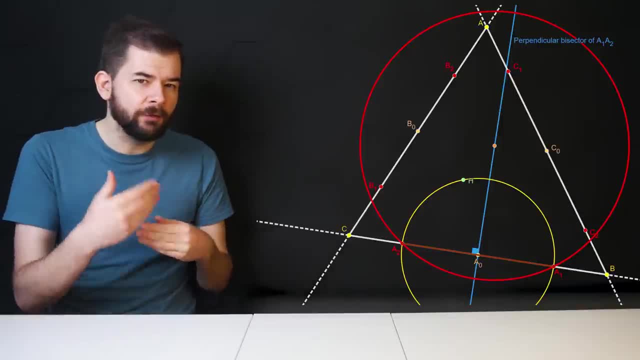 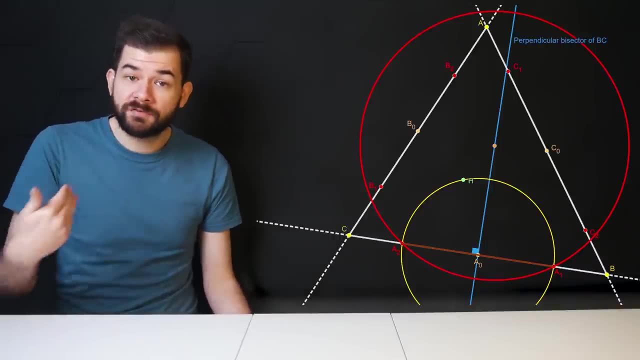 perpendicular bisector, which means that A0 lies on this perpendicular bisector, But recall that A0 is the midpoint of BC. thus, this is actually the perpendicular bisector of BC. We conclude that any circle containing A1 and A2 must be centred on the perpendicular bisector of BC. 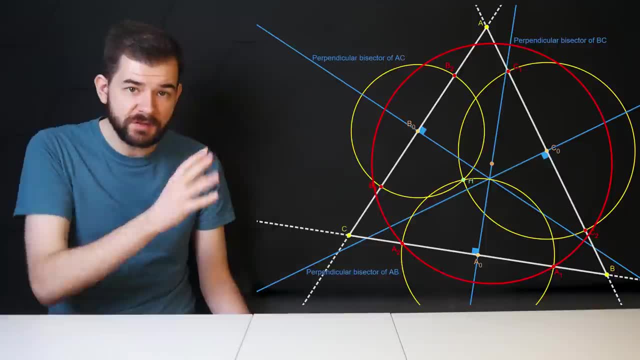 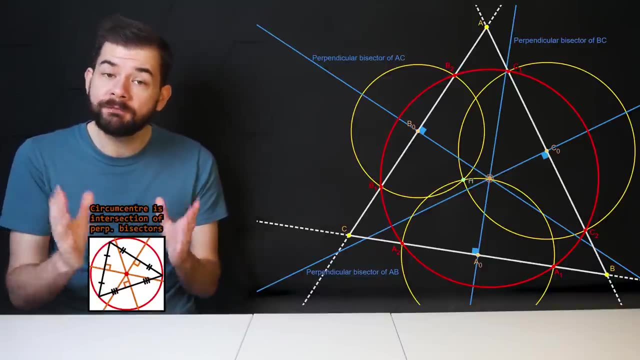 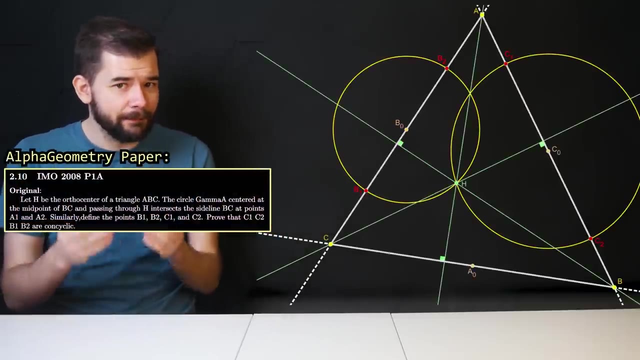 Repeating the argument for the other sides. any circle containing all 6 points must be centred where all three of these perpendicular bisectors meet, which is the circum-centre. So all three circles must coincide. So Alpha Geometry successfully solved this problem, which isn't exactly the same as stated in the Olympiad paper, and I don't like how the writers have simplified the problem. 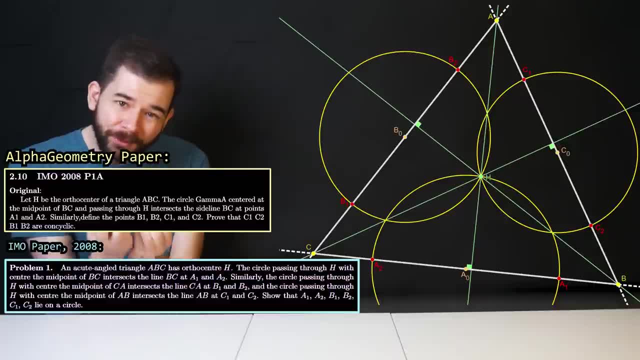 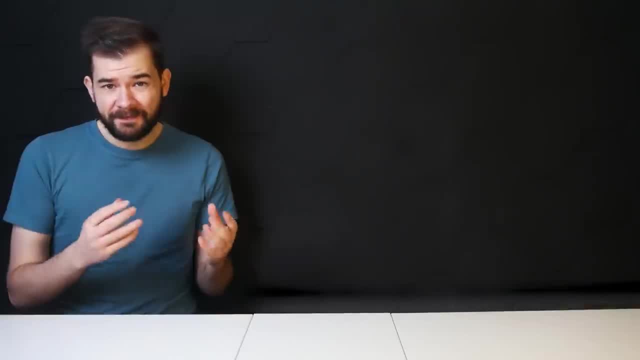 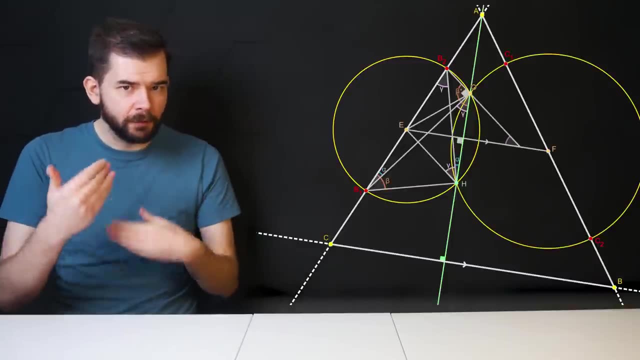 Yes, it turns out that it is a solution in this case, but that requires justification, and they haven't given any. The next thing to say about Alpha Geometry's proof is that it's quite meandering, to say the least. It isn't so much a solution, but more like watching someone else solve the problem in real time. 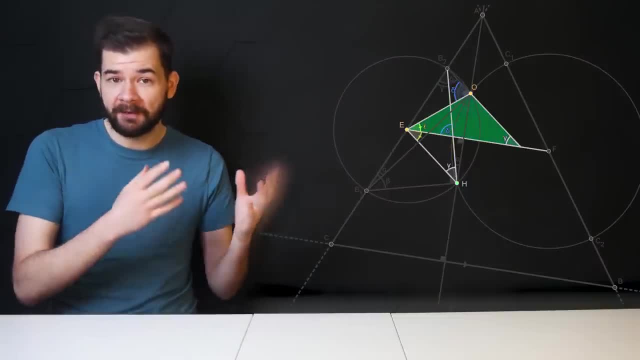 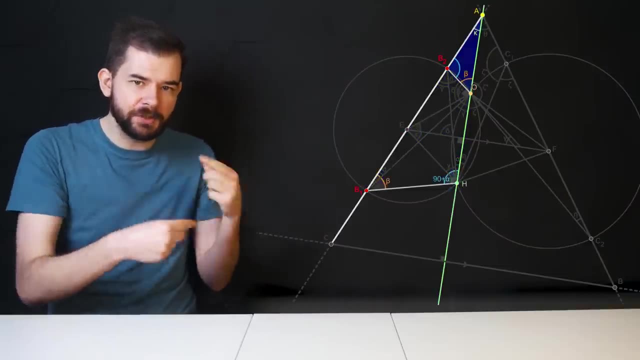 When we're solving problems, we don't always have the best idea first, so we tinker and meddle and hope that our ideas go somewhere. What I'd love to see is that if later versions of Alpha Geometry can refine the solutions into something more palatable. 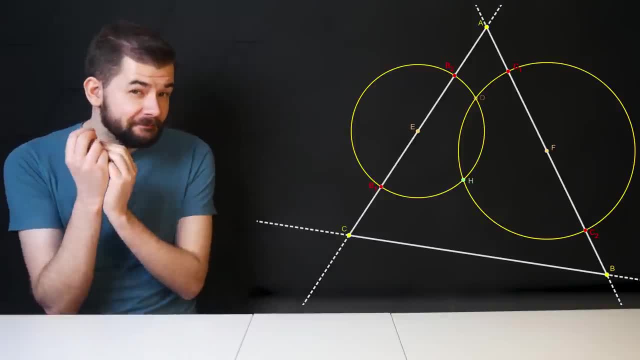 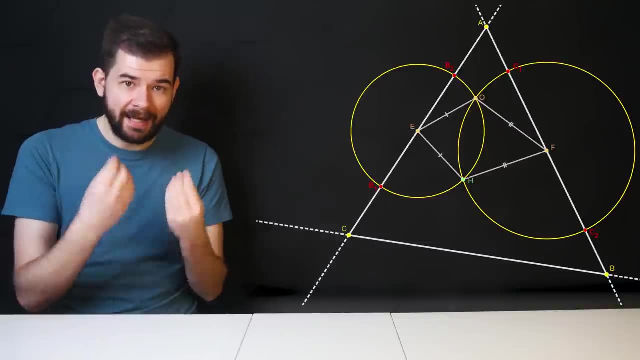 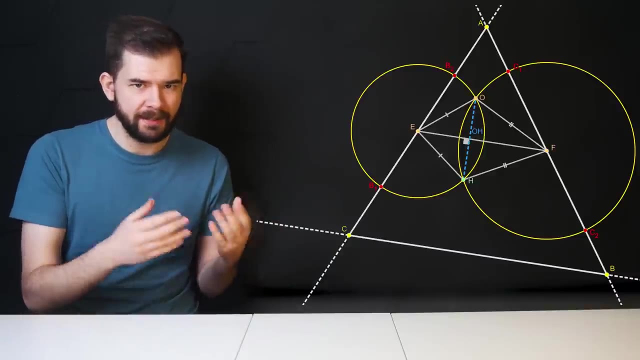 For example, consider this: Step 1, define O as the second intersection of these circles, And step 2, EHFO is a kite, so its diagonals OH and EF are perpendicular. This is well known, or provable in just a few steps, and if we can assume things like Saley's Theorem, I think we can assume this. 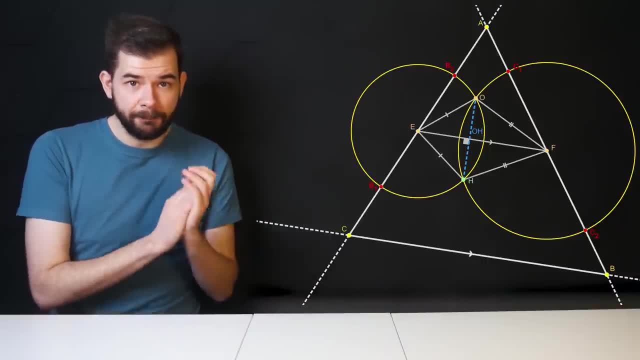 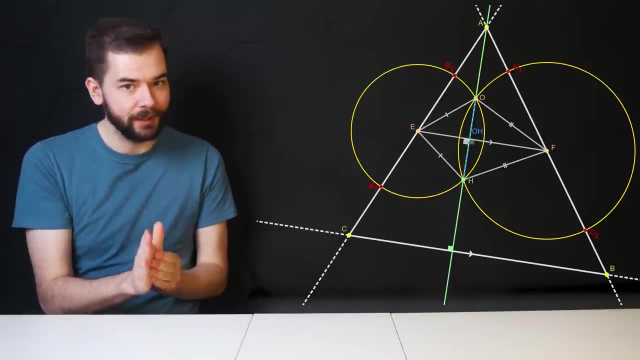 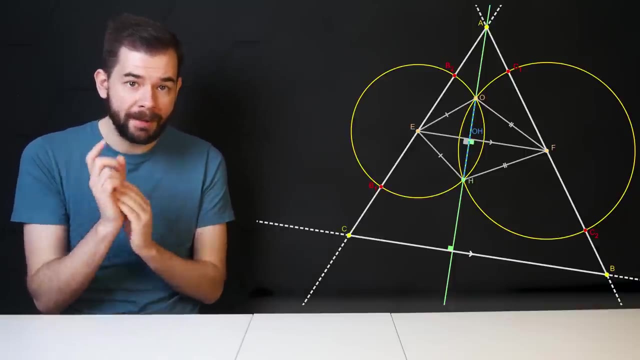 Step 3,, E and F are midpoints, so EF is parallel to BC And step 4, altitude, AH is perpendicular to BC by definition, which means it's perpendicular to EF. Since OH and AH are both perpendicular to EF, they are parallel and both pass through H, so in fact AO and H are collinear. 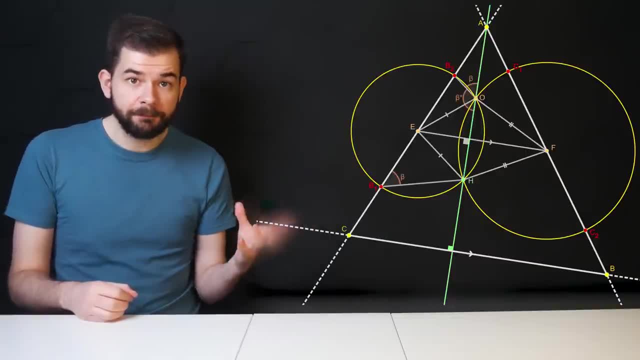 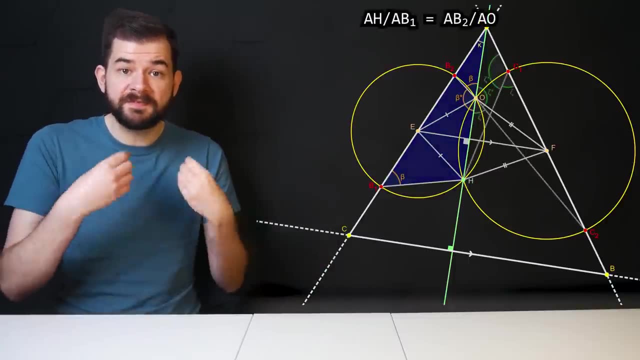 Steps 5 and 6 establish the betas as before, so these triangles with beta and kappa are similar, expressed as follows: And steps 7 and 8 establish the zetas, as before, so these triangles with zeta star and theta are similar, expressed as follows: 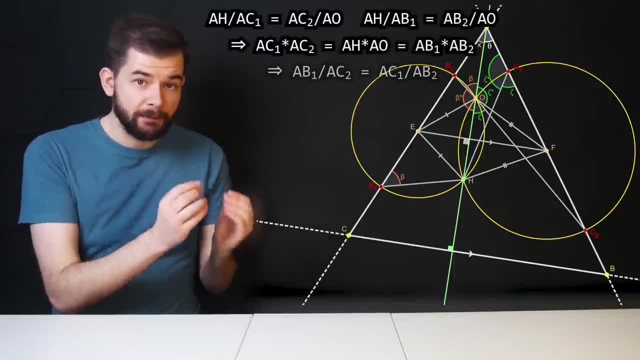 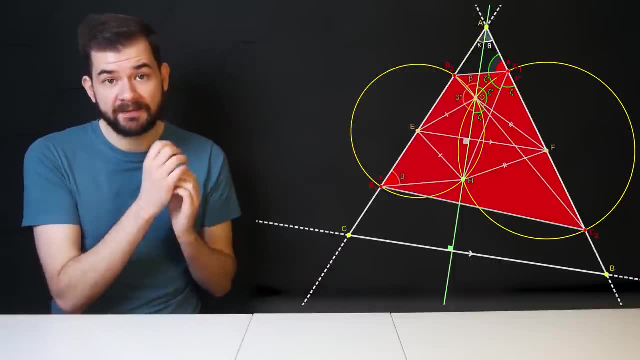 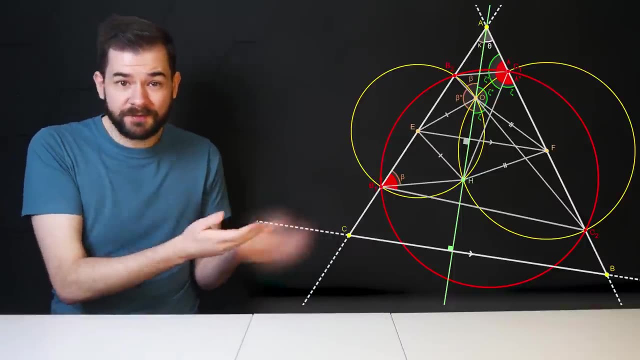 Steps 9 and 10 chase these ratios to establish similarity of these triangles, as before. Step 11 establish the lambdas, as before, And step 12 establish this quadrilateral as cyclic. And we're done. I'm sure we could shorten this further, but without much thought I took this from 40 steps to 12, with the benefit of hindsight. 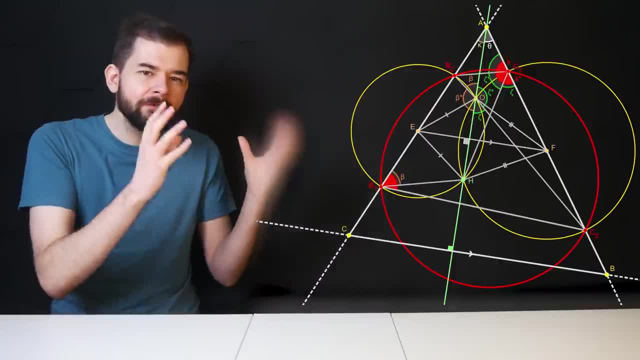 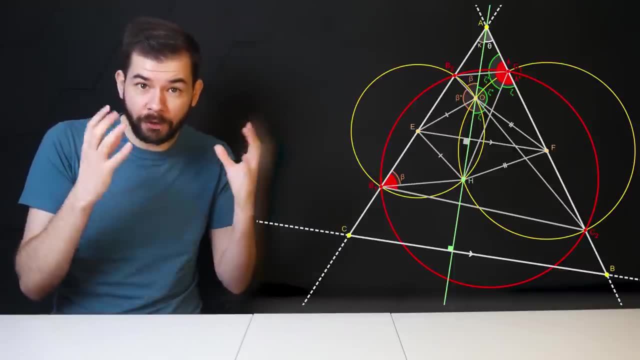 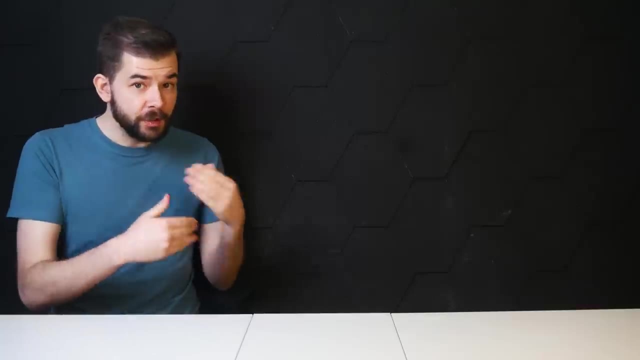 But my main issue with this proof is that the reason why the result is true doesn't leap out at me. A good proof should show why the result holds. The logic should enlighten us, And I don't find this particularly illuminating. However, this does veer close to my favourite solution to the problem. 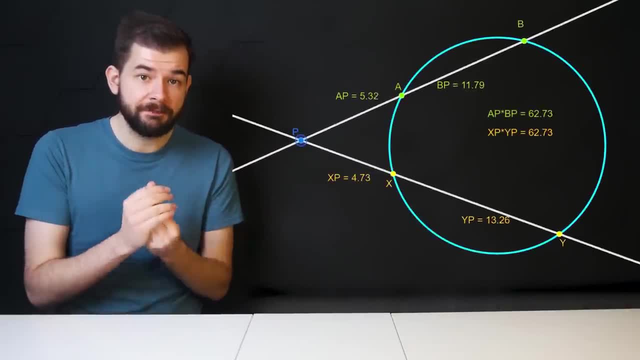 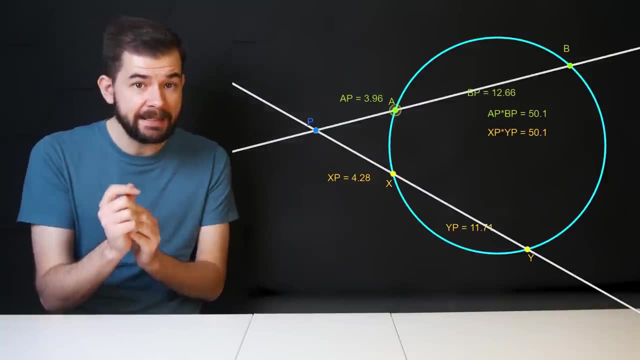 Consider the intersecting second theorem. This says that if you have two non-parallel seconds lines, one meeting the circle at a and b and the other at x and y and crossing at p, then the following holds: ap times bp is equal to xp times yp. 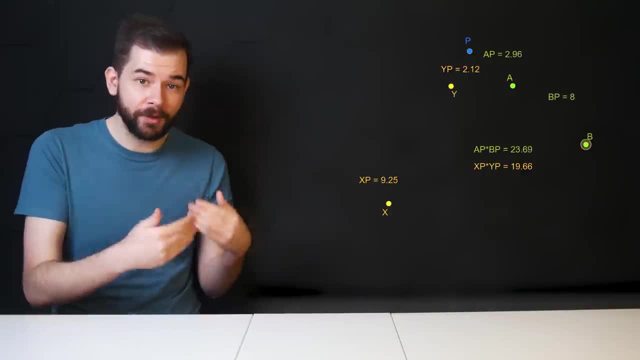 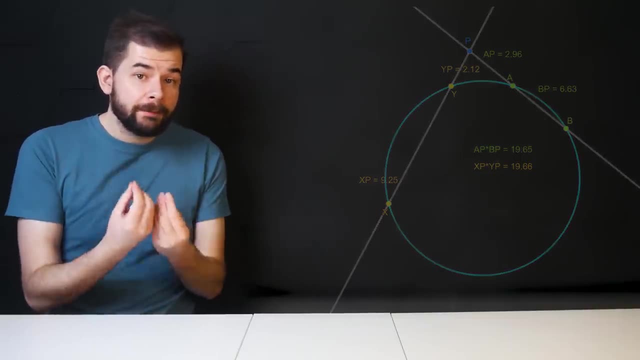 The converse is also true. If five points have this property, then those four points are necessarily cyclic. With that in mind, once we establish that a, o and h are collinear, we have, by the way, a, o and h are collinear. 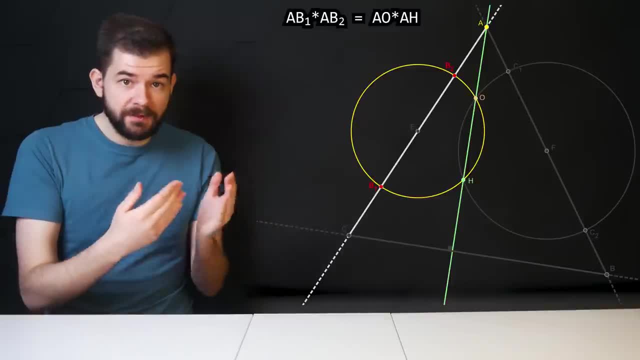 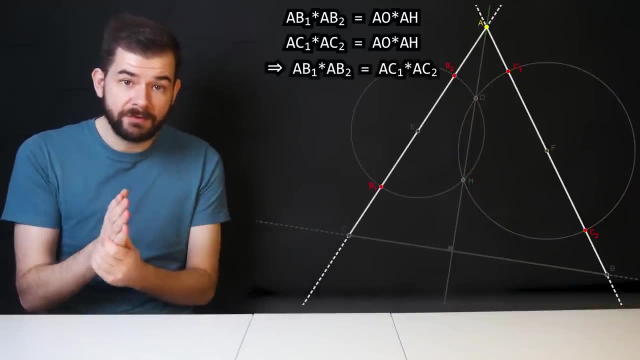 By the intersecting second theorem that ab1 times ab2 is equal to a? o times a? h, And ac1 times ac2 is equal to a? o times a h. Thus, ab1 times ab2 equals ac1 times ac2.. 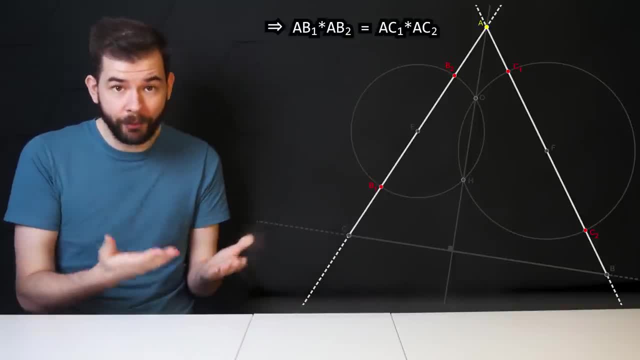 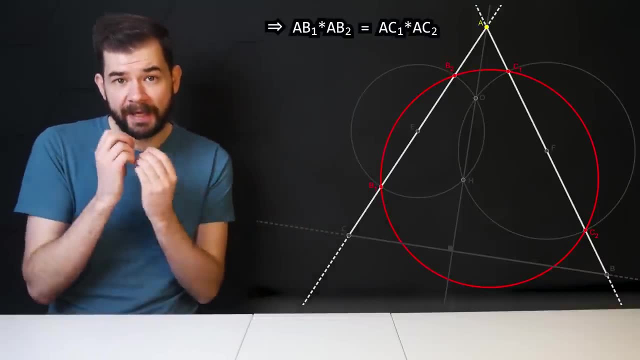 And by the converse of the intersecting second theorem. these points are cyclic. This proof was written by a human, and there is a wealth of other succinct and creative proofs out there. But, most importantly, this is a proof that, to me, 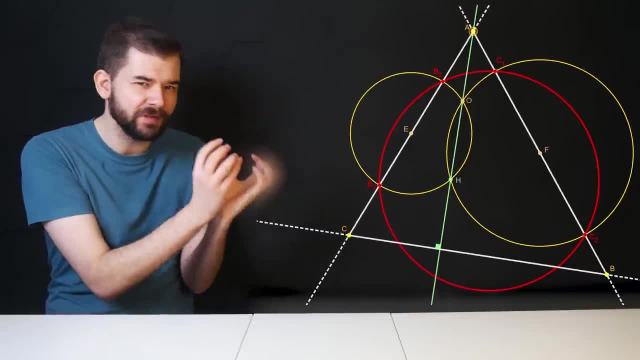 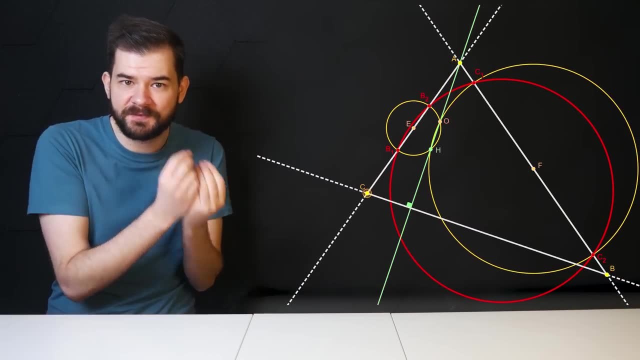 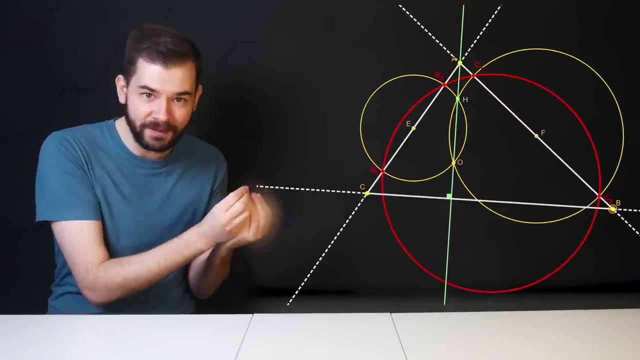 finally does the job. It does the job of telling me why the result is true. I can see it right in front of me: These seconds always combining at a vertex and therefore giving rise to this specific circle in the middle. All who love mathematics love the spark of insight that proofs like this give us. 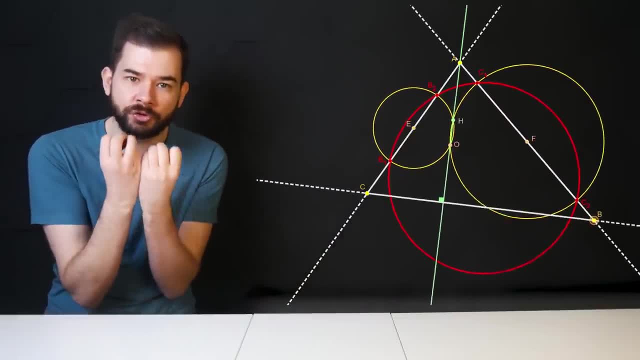 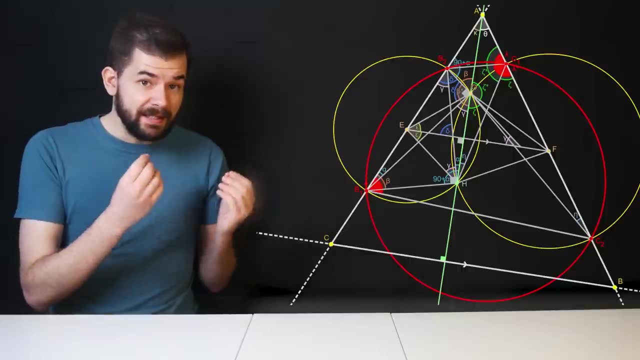 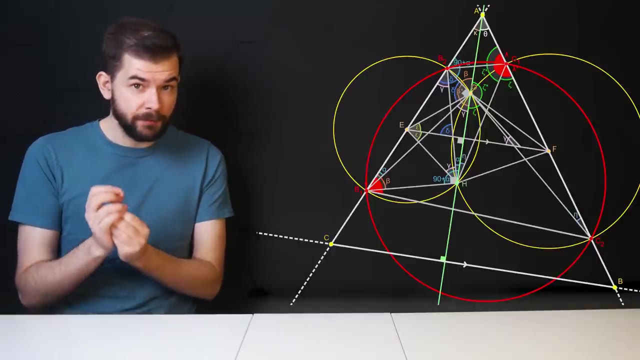 We don't want to just learn the results, We want to experience the unique joy of resonating with this kind of logical poetry. It's beautiful, This isn't, But is that a problem? After all, it got the answer, and it did so in this unique way of combining creativity with deduction. 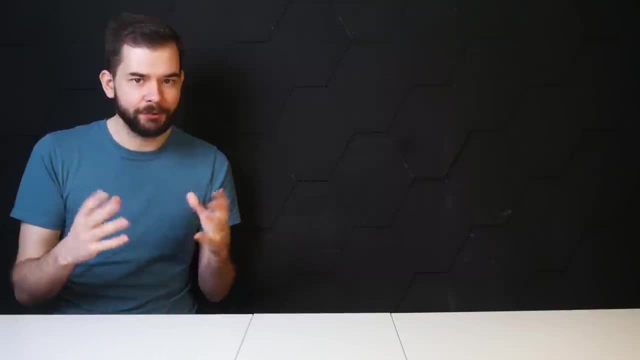 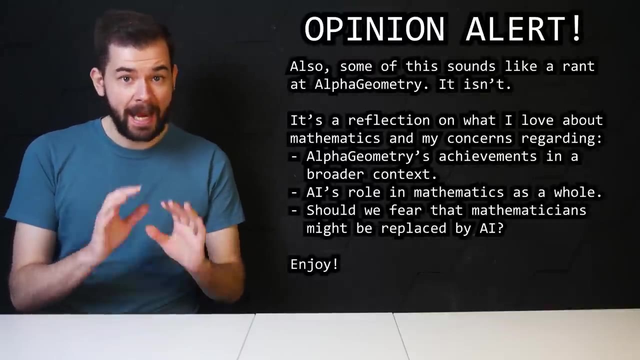 So let's now take a broader look at what I think alpha geometry means for AI and what it means for mathematics. Let me just remind you that I am not a computer scientist. I am a mathematician first and foremost. Everything that follows in this video is just like my opinion, man. 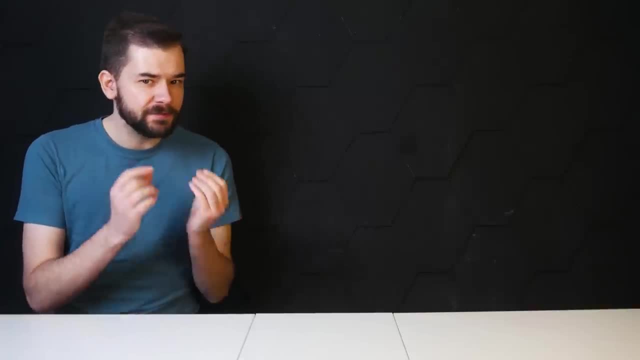 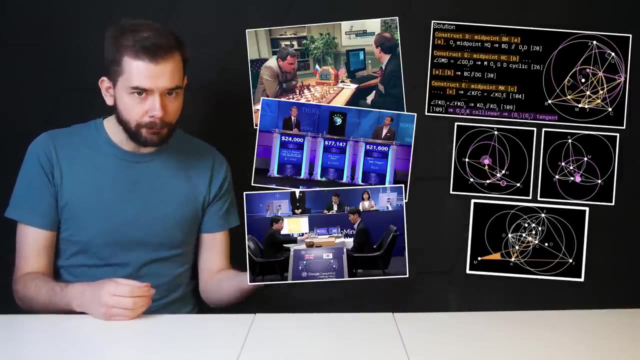 Let me loop back to something I said at the start of the video. The previous AIs learned to play games, while this one can solve problems. Well, is alpha geometry really solving problems? Because it looks like what it's doing is brute-forcing its way around the angles and eventually landing. 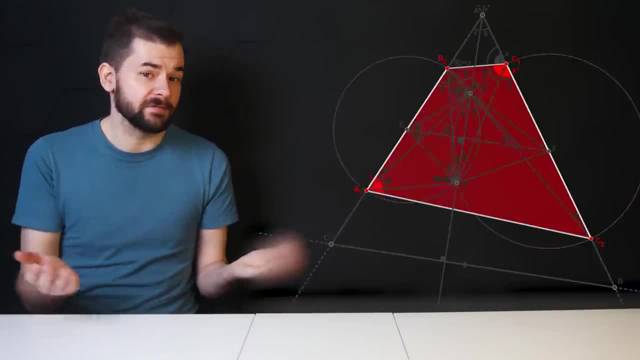 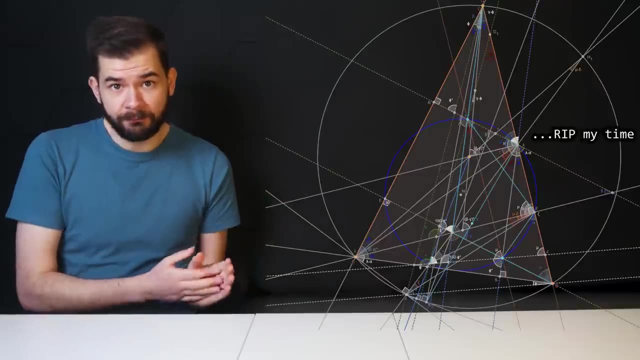 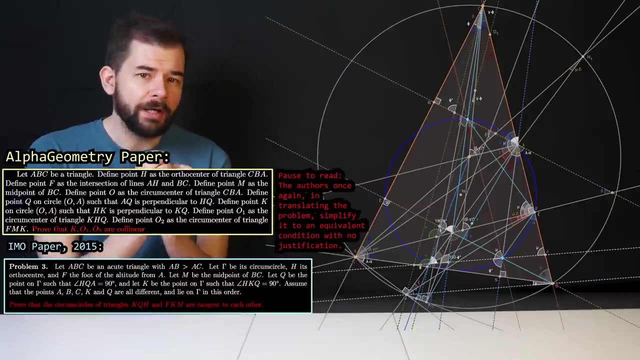 on the result, But isn't that what problem solving is? Alpha geometry solutions are pretty haphazard and lacking in any general direction. Look at this solution for problem 3 of 2015's IMO- Horrendous, But if you try these problems, what do your initial attempts look like? 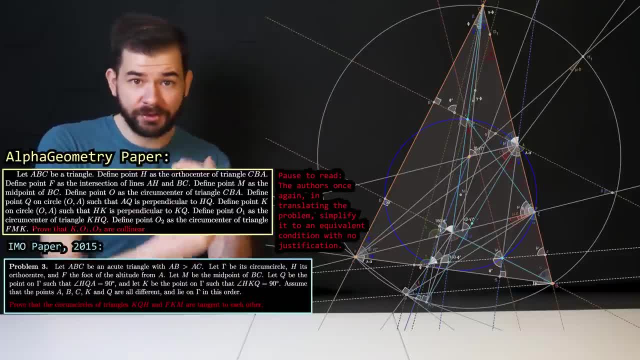 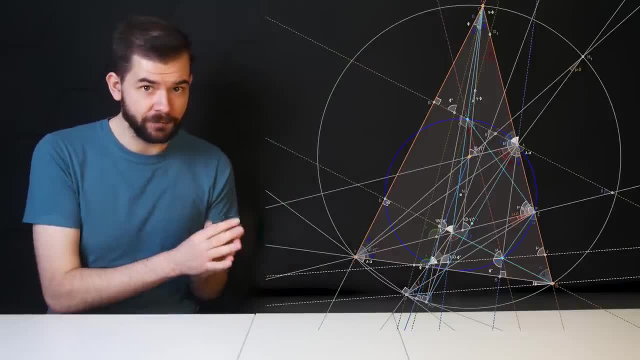 I think for most of us we just get confused. We just get our hands dirty and work out a bunch of lengths and angles before we have a good idea. We might have slightly more direction and intent behind our choices, But is our approach radically different to alpha geometry's? 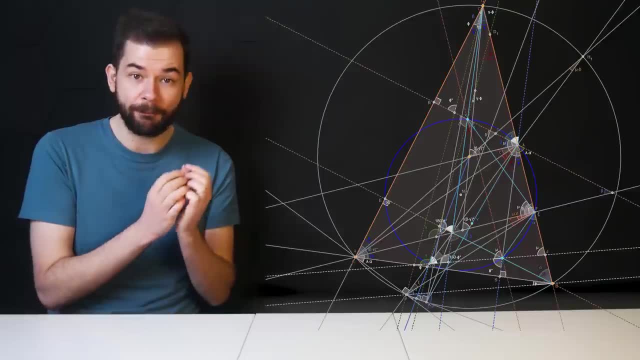 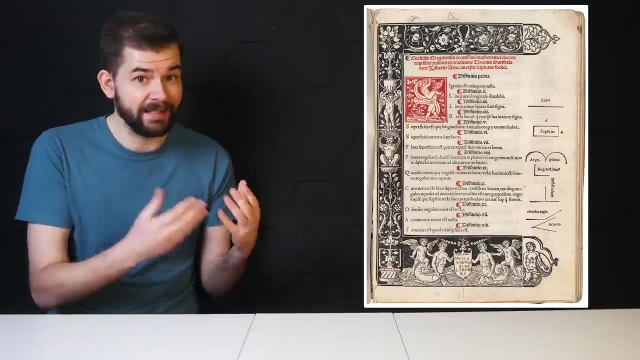 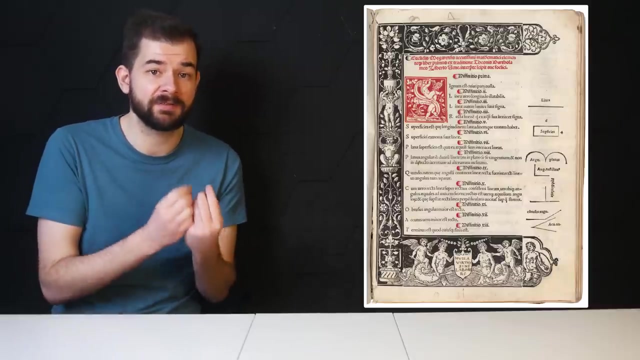 I don't think so, And I find this aspect of alpha geometry impressive and fascinating. A less impressive aspect of alpha geometry is that plain geometry is easy to codify in terms of strict rules and results. I mean, The oldest recorded axiomatic approach to mathematics is Euclid's Elements and that. 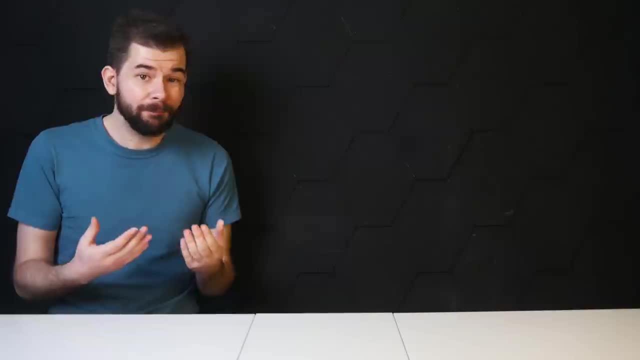 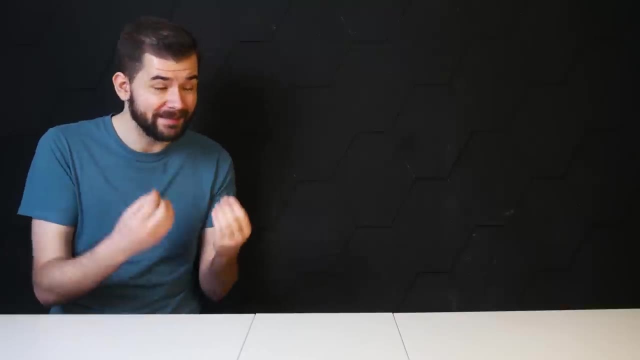 begins with plain geometry. Olympiad problems are kinda like games: We know they have an answer. We know they are solvable with high school level results because that's how they are designed For the language model, right brain. there are only certain things you can try and certain. 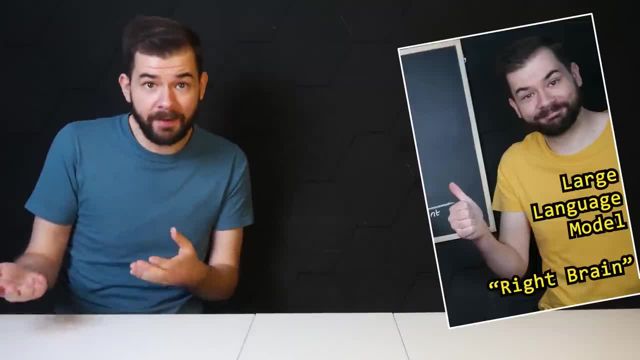 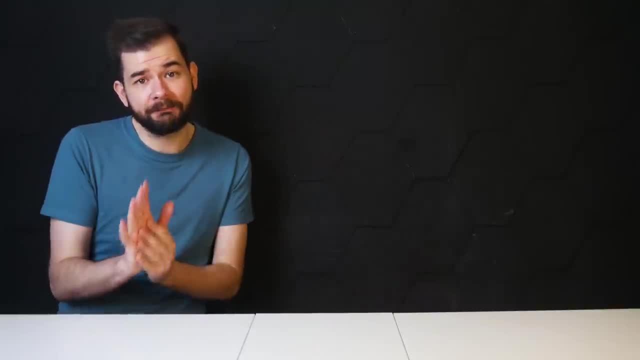 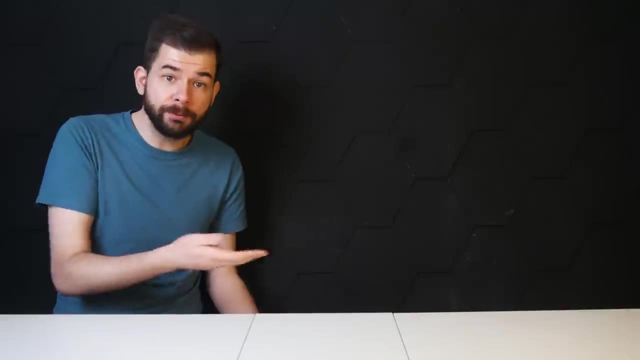 things you need to try. Compare this to analytic number theory or algebraic geometry, where problems demand ideas that are way out of line. This is to say that I don't think alpha geometry's achievements can be immediately generalized to other fields of study, no more than chess computer Deep Blue could attempt. 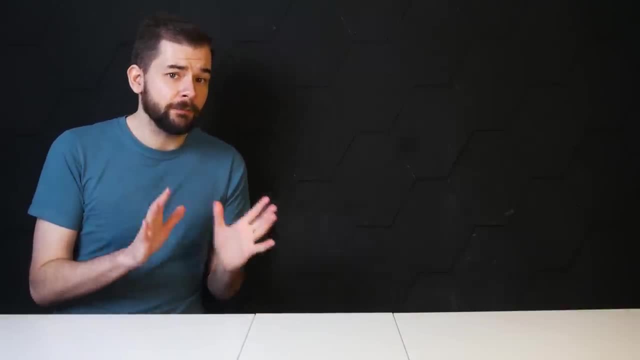 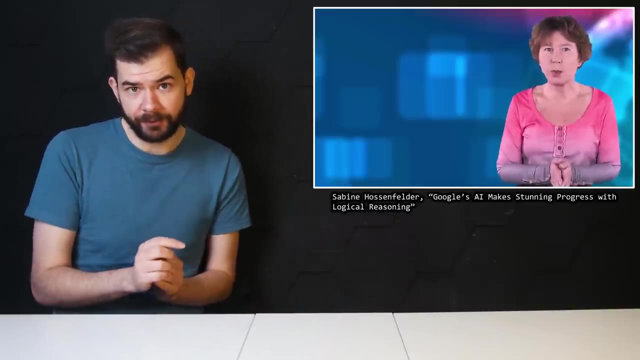 to play Go. It's for this reason that I respectfully disagree with some other commentators on this topic. Sabina Hossenfelder, for example, had this to say about alpha geometry: It generally highlights AI's growing ability to reason logically, discover new knowledge. 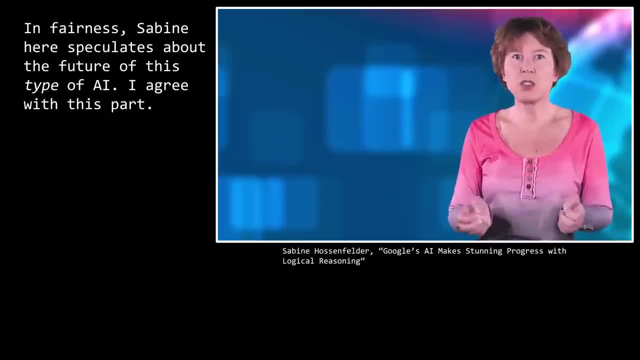 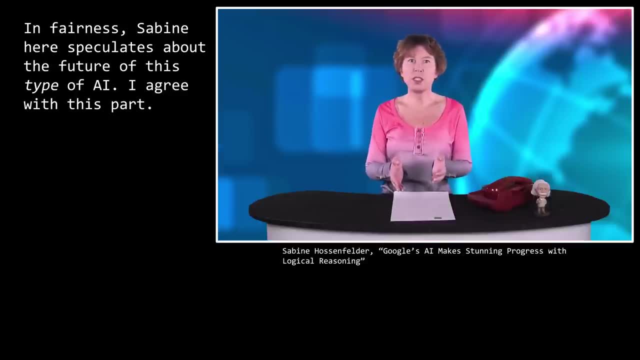 and verify solutions. And not only this, it can also explain how it arrived at a conclusion. Such a type of AI system has uses that extend beyond geometry. Not only can this achievement be generalized across various mathematical domains, but it'll without doubt also come in handy in other areas where rational thinking and logical 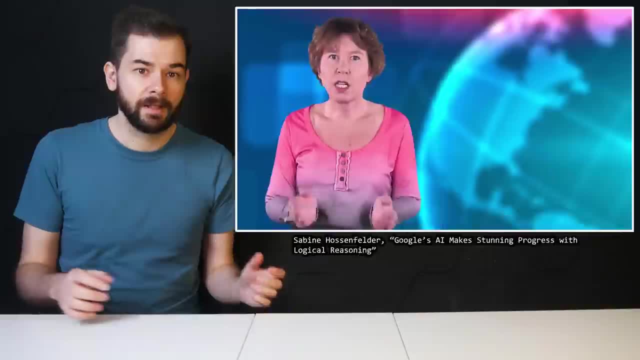 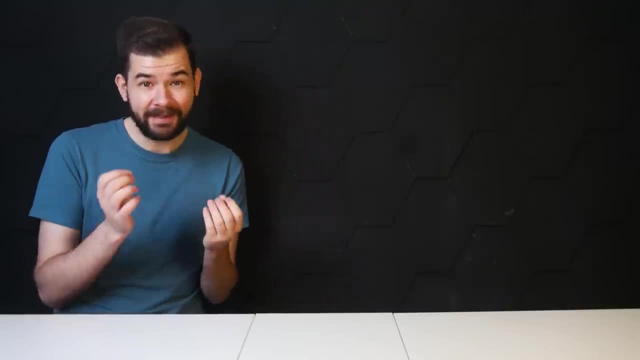 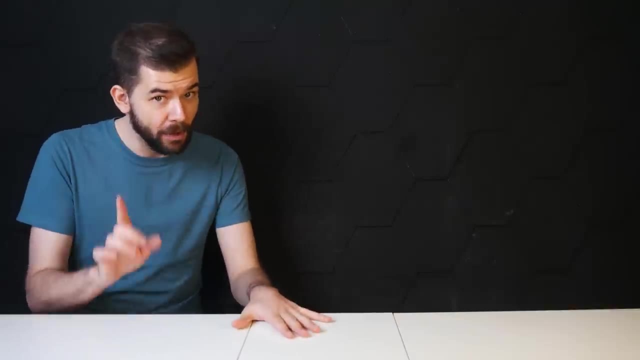 deduction is of use. Like everything High school level, plain geometry questions which, remember, are written to be solvable, are comparatively easy, and there is currently no evidence to suggest that this technique can be generalized at this present time. Now, I'm not so naive to think that things will be different in the near future, especially. 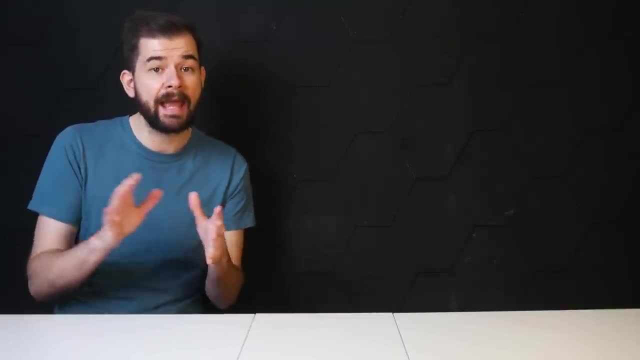 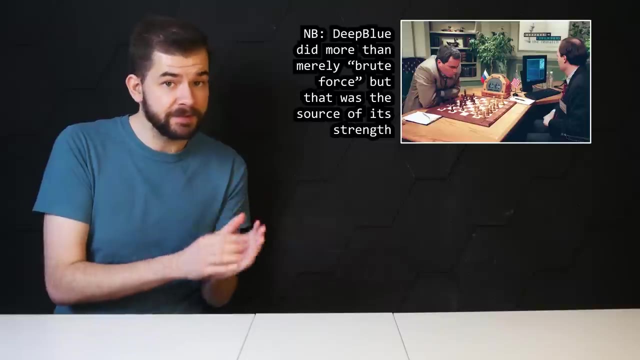 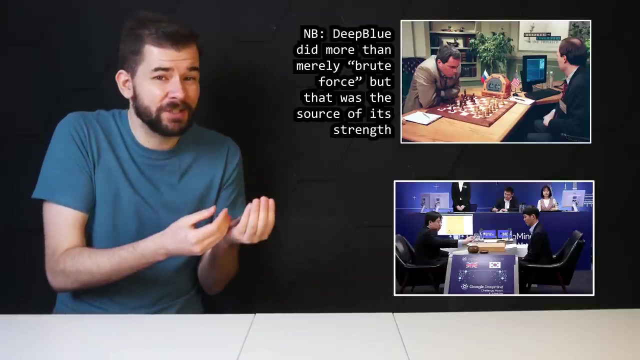 given the rate of AI progress, So maybe soon an AI can tackle something like algebraic geometry, but not right now. A computer brute-forced chess, but it still took 20 years before a computer won at Go. Here, alpha geometry is answering geometry questions by 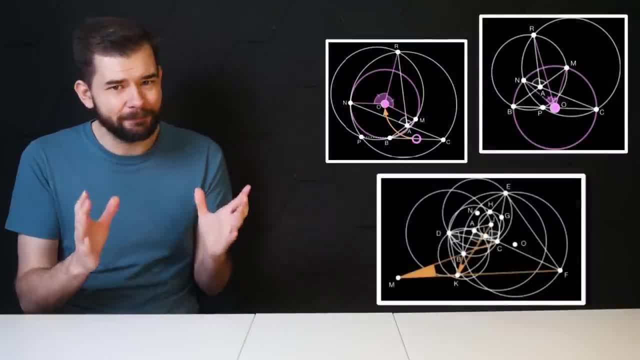 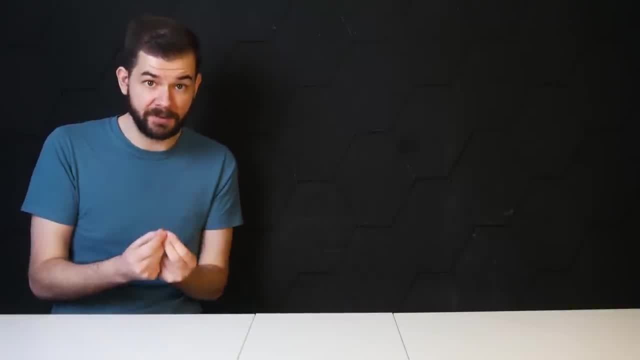 Well, not quite brute force, but it's similar And I think that we're still a while away from seeing AI have a go at some of the unsolved problems across mathematics. And come to think of it, given all the operations alpha geometry can do every second, it's still 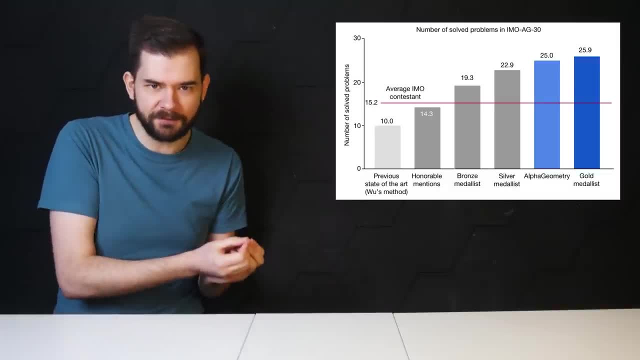 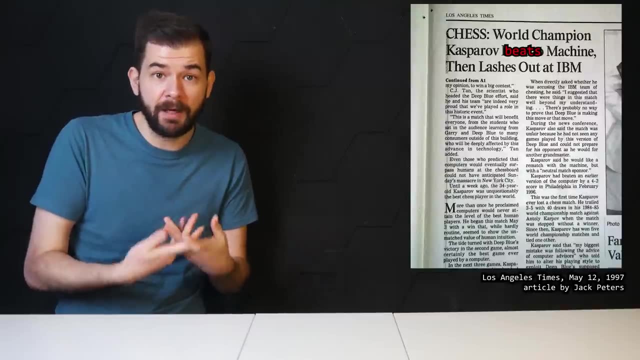 surprising to me that it still can't outperform the best humans. How weird would it have been if IBM announced that its computer Deep Blue attempted to beat Garry Kasparov but came second? No, The victory over the champion. What The champion was the milestone. 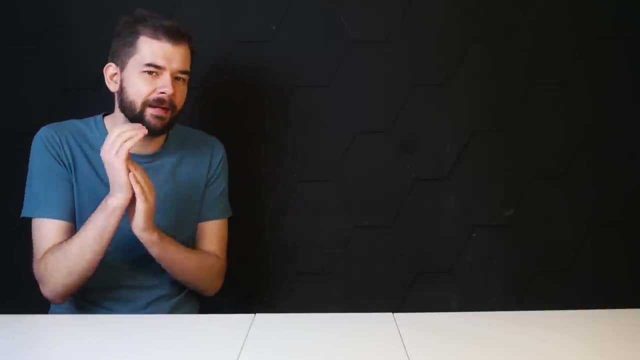 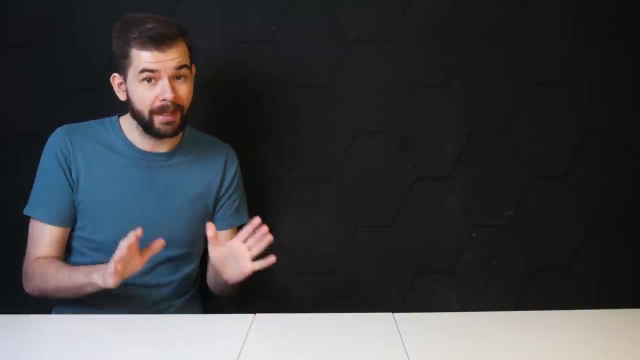 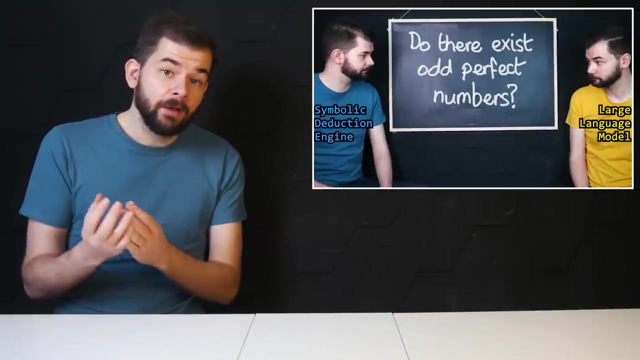 I'm not taking away from the achievements in this paper. I just think our excitement should be tempered a little. In my mind, this is a small step beyond beating games like Go, not a radical leap forward. It's natural, then, to ask about the future and whether AI will tackle unsolved problems. 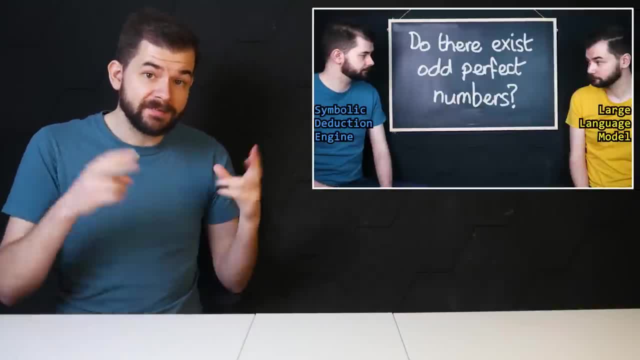 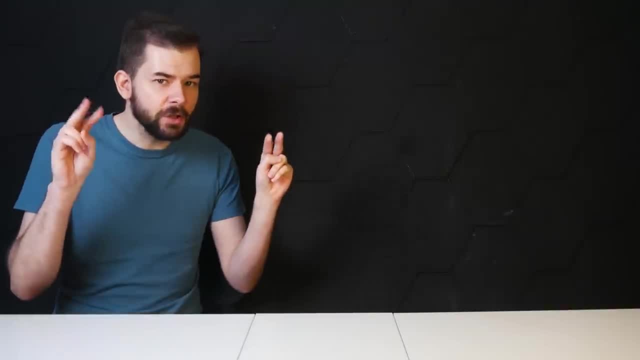 Those of you who have read the paper will know that alpha geometry developed many synthetic theorems, results proved from its foundation that help it make inferences. It even discovered a new result in this question because its solution doesn't require one of the premises. 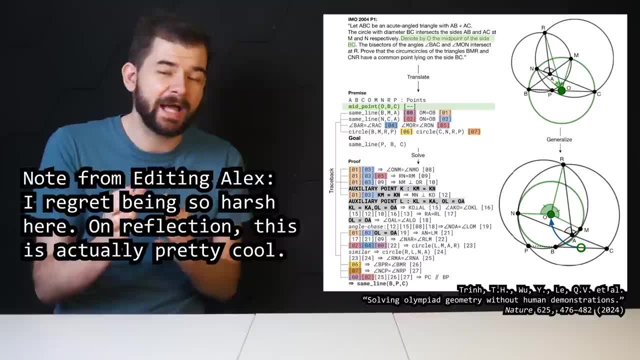 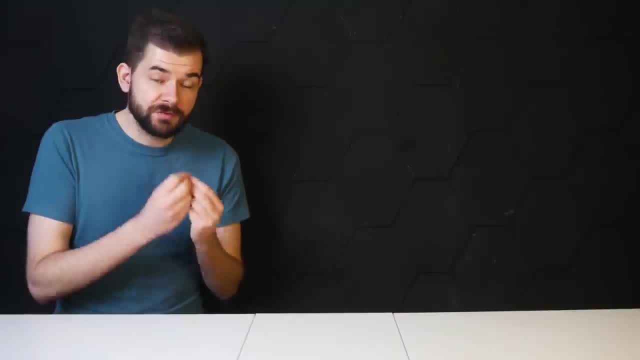 I'd be gobsmacked if the question setters didn't already know about this and just added this constraint to tune the difficulty of the question. But is this a sign of AI eventually being used to solve open questions, And is that a good thing? 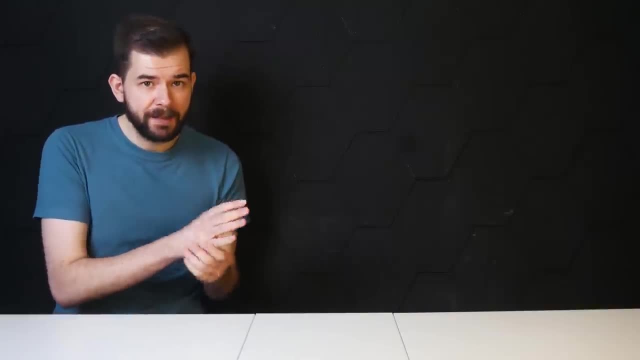 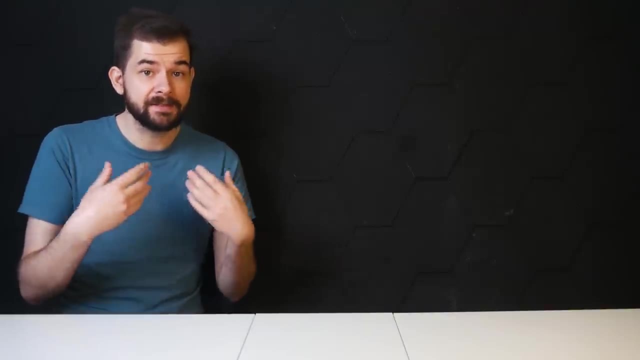 Well, the first thing I foresee is AI-assisted proofs. These fall into a similar region of computer-assisted proofs, but there might be a difference. Computer-assists are basically AI-assisted proofs. The four-colour theorem, for example, required a lot of pen and paper research to break down. 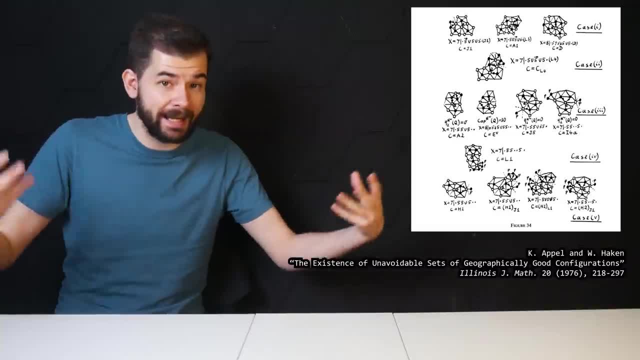 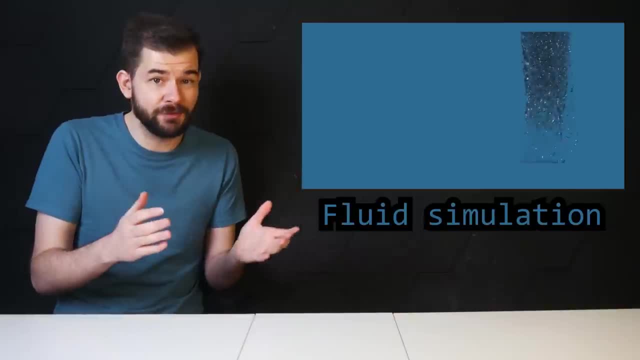 the number of cases, each of which could then be checked by hand, but a computer can do it much faster, so it's more practical. Even simulations and data analyses essentially boil down to just doing a lot of calculations, which could be done by hand if we had infinite mathematicians writing on infinite blackboards. 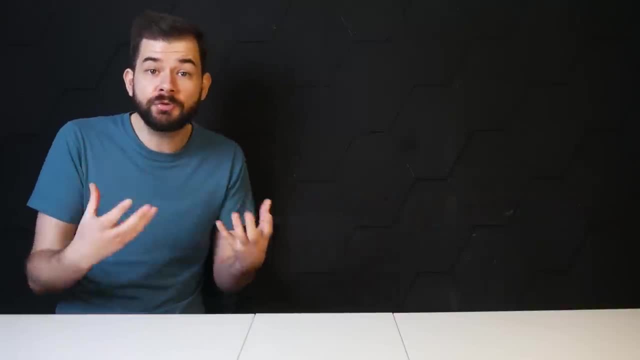 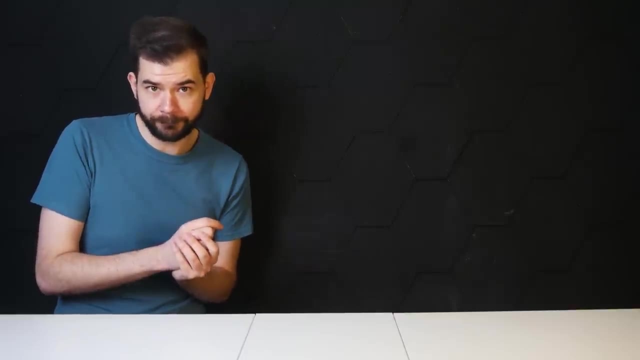 but we do it by computer to save time. A computer is just part of the equipment of the modern 21st century computer. It's not just a computer, It's a 21st century mathematician, along with chalk and blackboard. 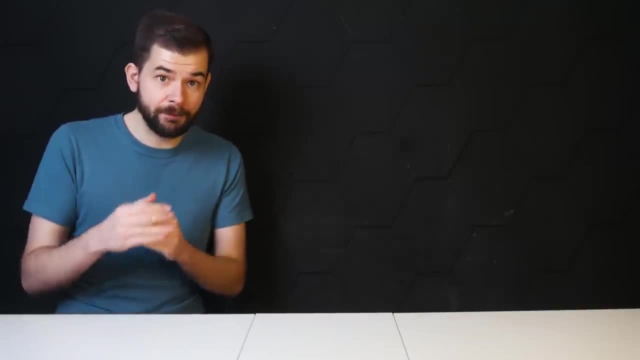 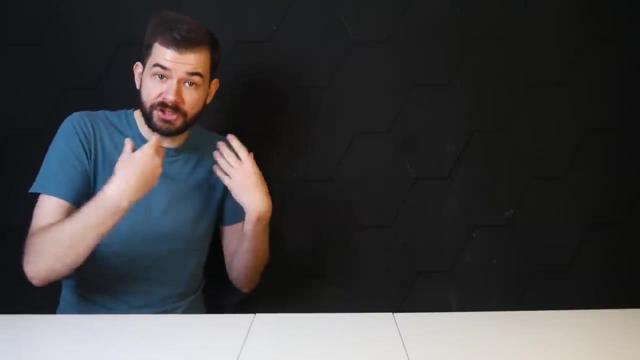 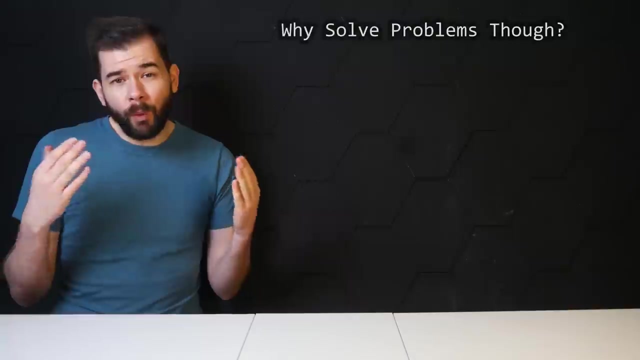 Along with traditional computer assists. AI assists might be considered part of our toolset as well, but AI might replace some of the creativity involved, and so would a purely generated AI proof. It feels like cheating, But is that a bad thing? Well, we need to ask. why do we bother solving hard problems? 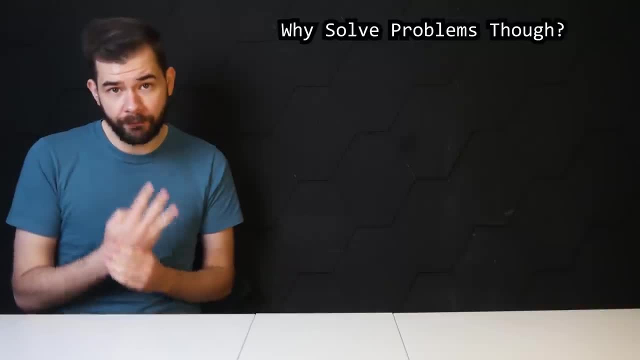 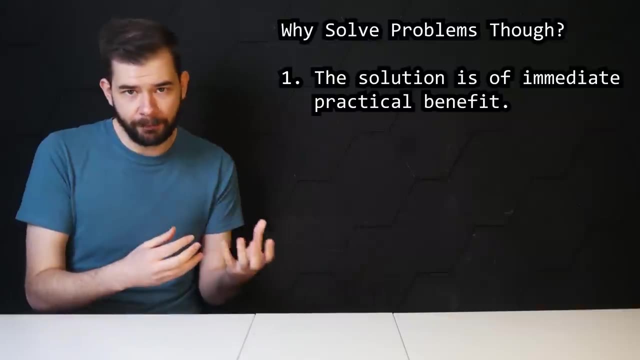 Other than to satiate our curiosity. I think there are three reasons. The first is that they have immediate practical value. These are things like optimisation problems that could revolutionise aspects of computing, Or cracking the Enigma code. It shortened the war. 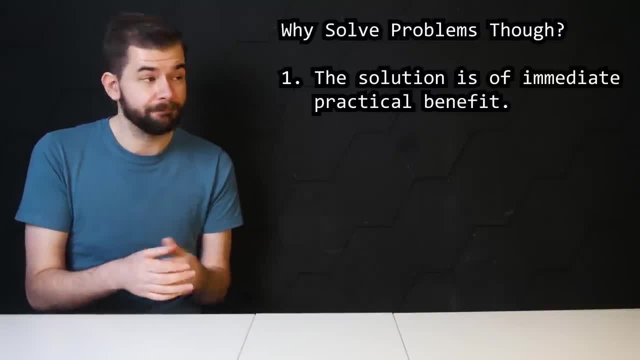 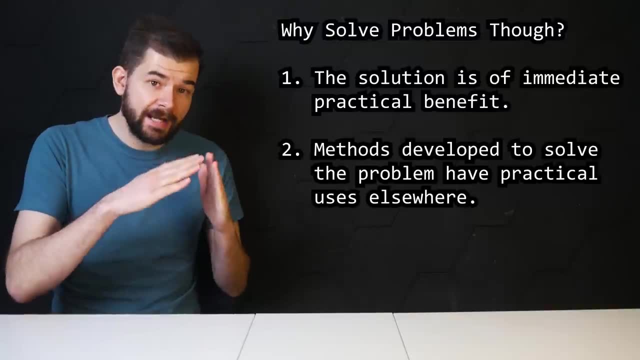 Direct impact. A non-mathematical example would be curing a disease. It's just good. The benefits are immediate and tangible. The second reason is that the theory or techniques we develop in order to solve them could be used elsewhere. This is the spin-off effect. 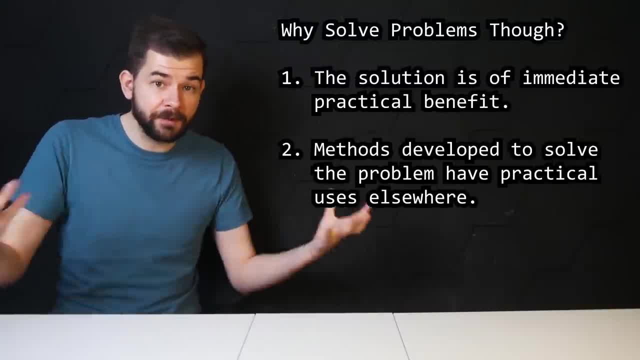 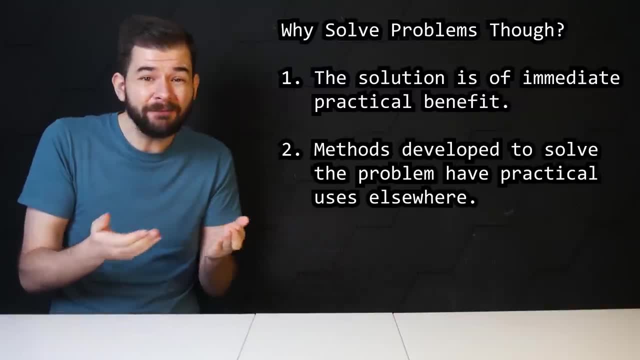 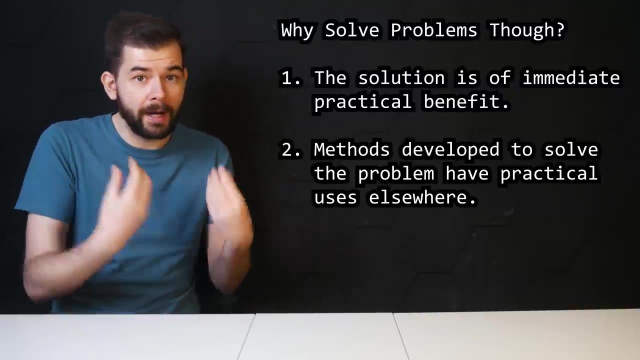 Proving Fermat's Last Theorem, for example, required several leaps that connected many areas of mathematics and improved our overall understanding. A non-mathematical example might be that we didn't really gain any practical value from Armstrong setting foot on the moon, but many innovations were required to get him there. 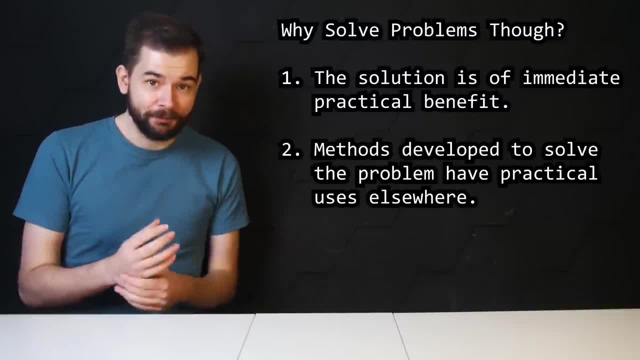 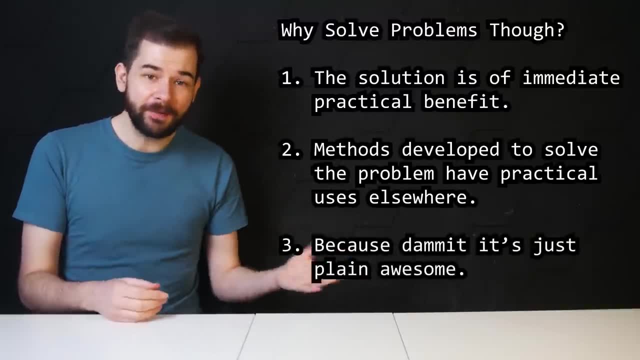 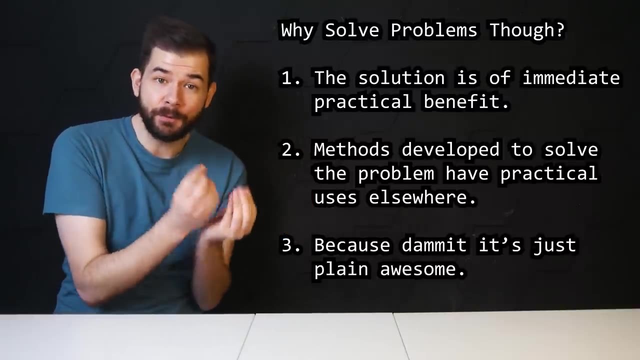 which have everyday use. Thirdly, most importantly for me as a pure mathematician, and a reason I think is overlooked, it's just good to solve problems. You know Why climb Everest? Because it's there. Even without the innovations required for the Apollo missions, I still find the moon. 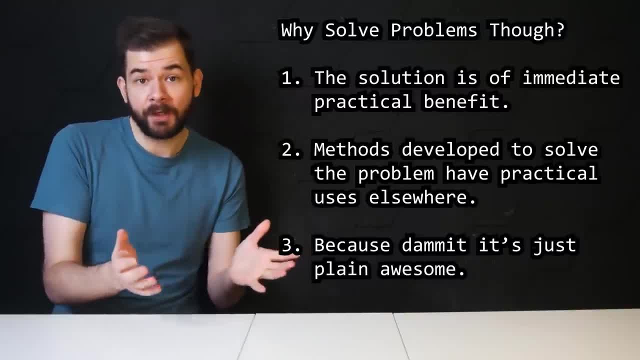 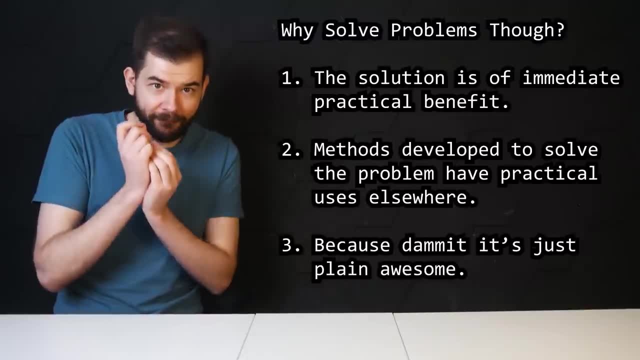 landing endlessly inspiring. Maybe the proof of the Collatz conjecture won't directly impact my life in the slightest, but I'll still find the event enormously inspiring nonetheless. Basically, the reason we solve problems, and really the reason we do anything, is either: 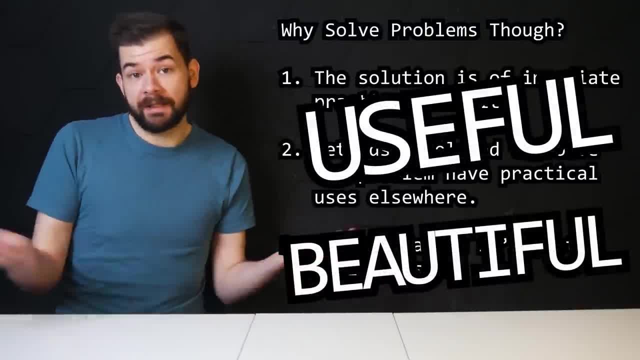 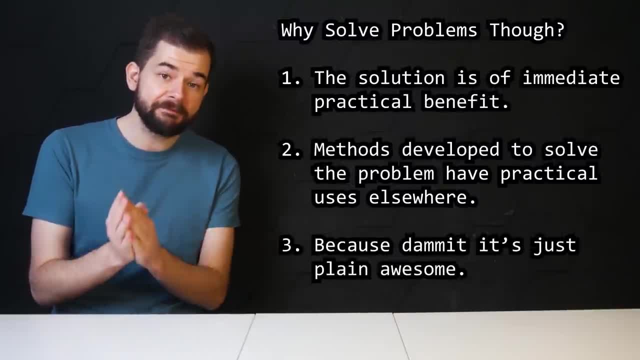 because it's useful, or because it's beautiful, Or it's neither- like my PhD thesis, But still Reasons are valuable. So here's my take on AI in mathematics: If a solution to a problem has immediate practical value, we should use AI and cheat. 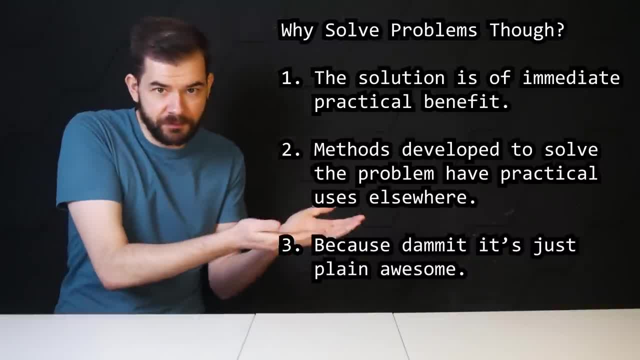 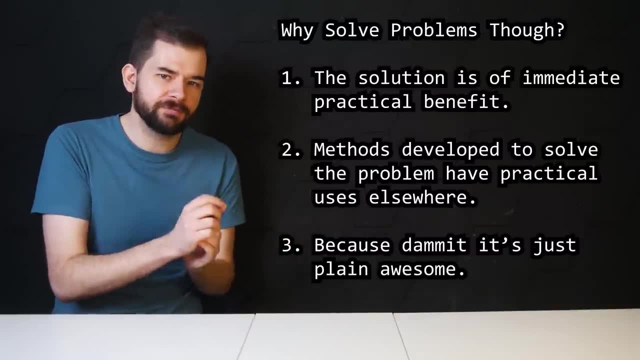 and get the answer. Who cares if we look up the answer to a disease cure, It'll save lives. The second case gets a bit weird, though. I worry that AI-assisted proofs might not develop interesting spin-off theory and instead force the solution out of pre-existing knowledge. 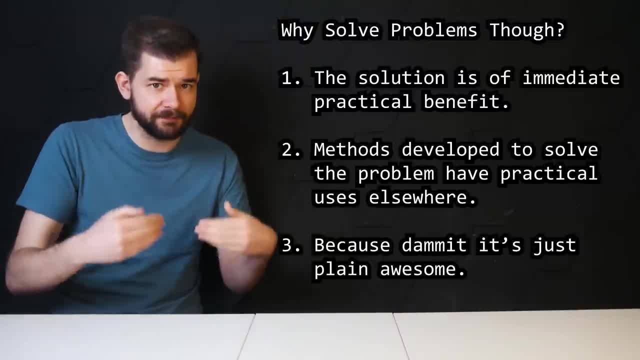 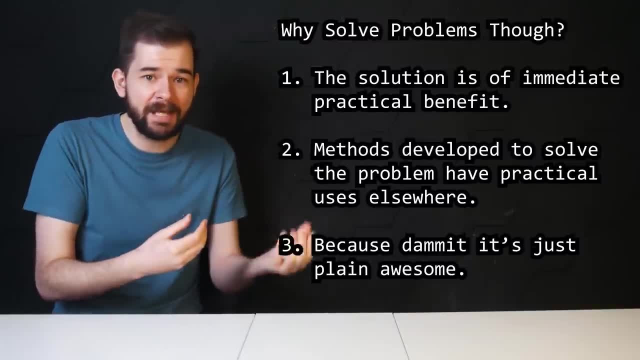 When humans puzzle for a long time, they force themselves to be creative, and that's where the new theory lies. AI might get the answer with a messy and haphazard application of more basic stuff, so we miss out on potential new techniques. 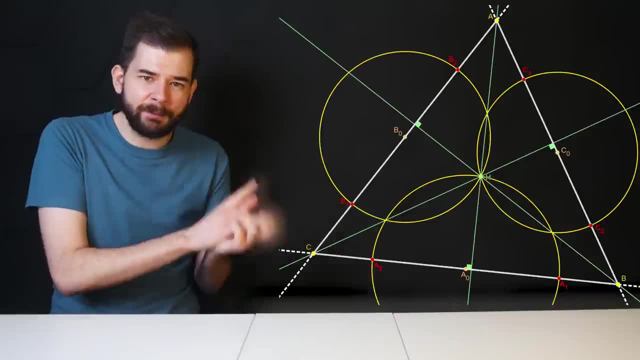 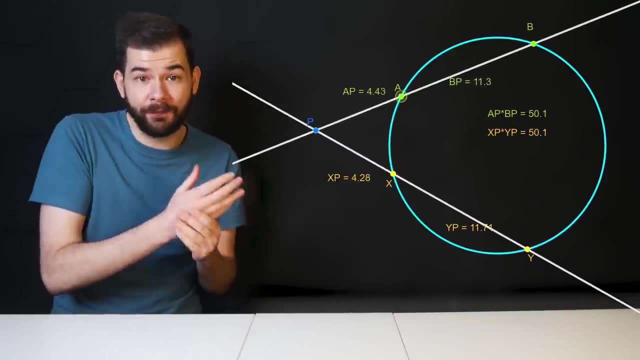 This isn't exactly the same, but by analogy it's like this geometry problem. Did you know the intersecting second theorem before you saw this proof? You might have done. but alpha geometry, on the other hand, applied the same few results over and over. 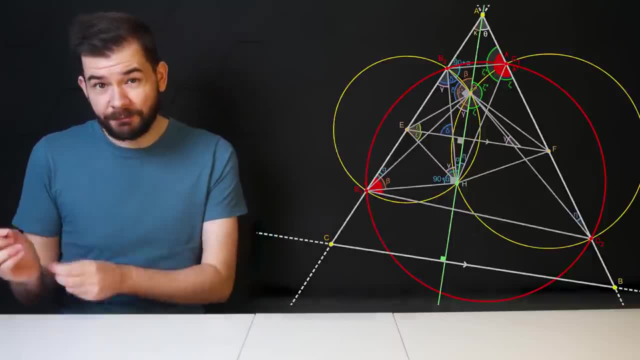 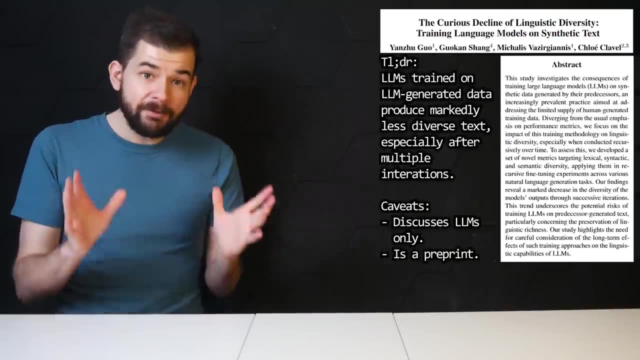 Admit it. Admittedly, that's just my opinion. I don't really have any direct evidence of this, but we are already starting to see stagnation in other areas of AI-generated content. But my main reservation with AI-generated proofs is this third point: the beauty. 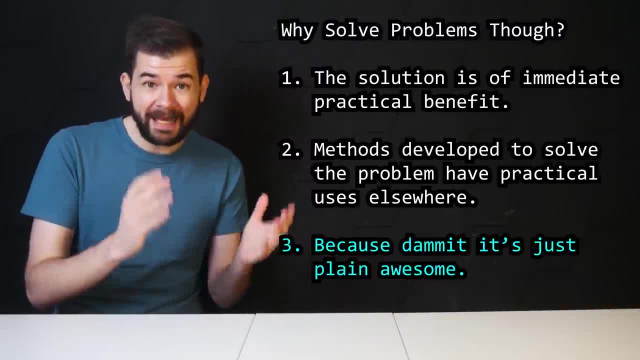 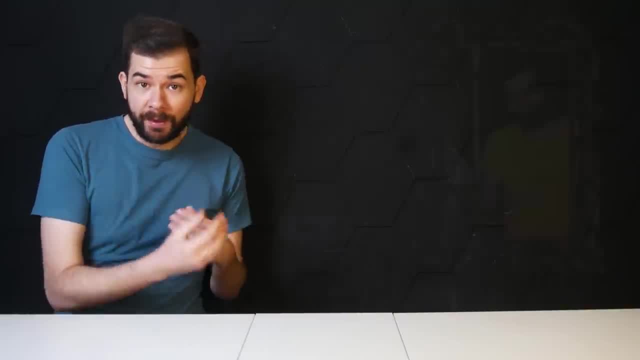 I know alpha geometry wasn't designed to create beautiful proofs- and again, this is just my opinion, but I want to convince you why beauty really matters. Imagine if an artist composed the greatest painting ever. There is likely no practical value to be found in the painting. 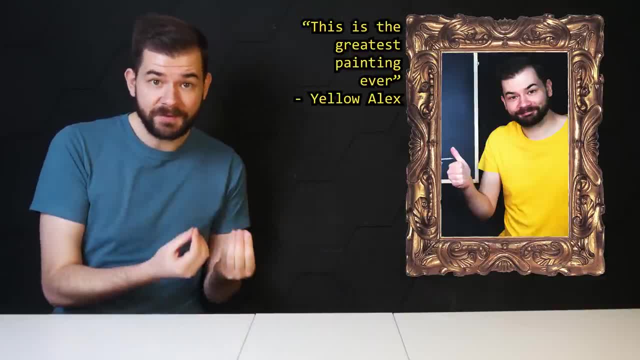 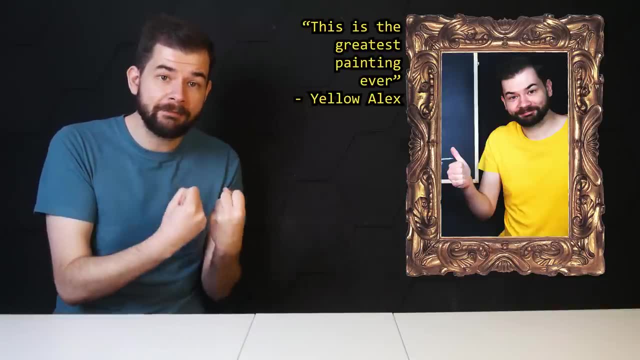 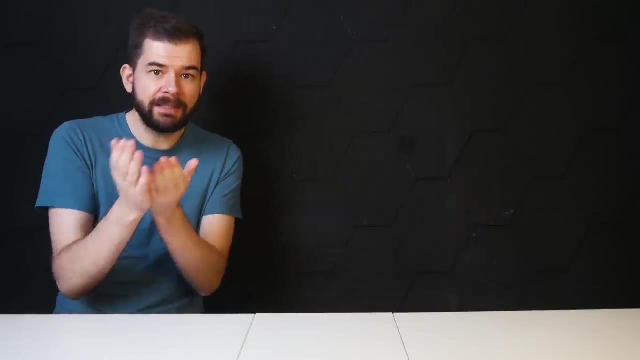 Or in any of the techniques developed to compose it. but we wouldn't say that it's pointless. As an enormous cultural contribution, it would still enrich our lives in ways beyond what is practical. Well, mathematics is part of our culture. Has your life tangibly and practically improved because Wiles proved Fermat's Last Theorem. 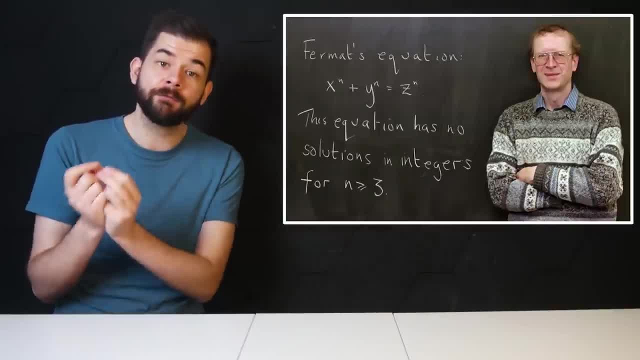 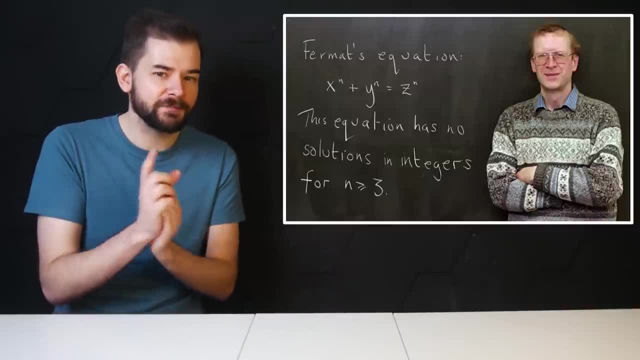 Probably not, But the story likely inspired you. The result was as much an enriching cultural contribution as a great piece of art. I hope you enjoyed this video. Would the story have inspired you if an AI had proved Fermat's Last Theorem? 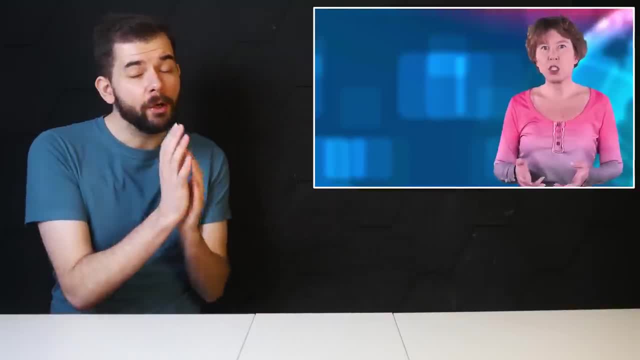 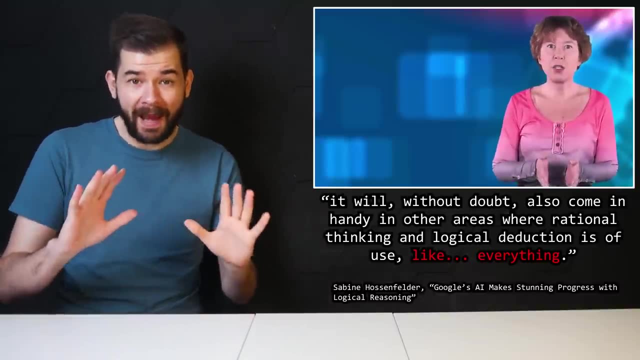 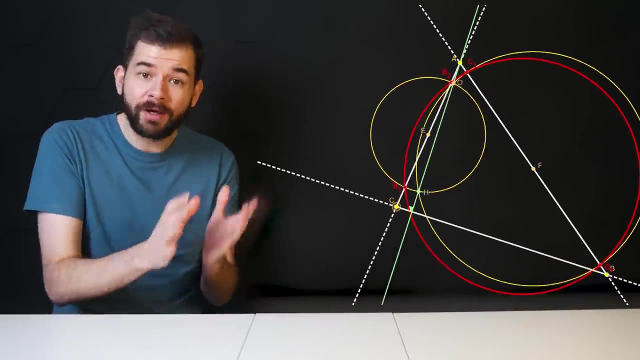 This is again where I disagree with Sabina. I know this last comment was a bit of a joke, but rational thinking and logical deduction aren't useful for everything. I can't rationally convince you why this proof is beautiful To me, it just is. and nor can I convince you why alpha geometry's proofs are ugly. 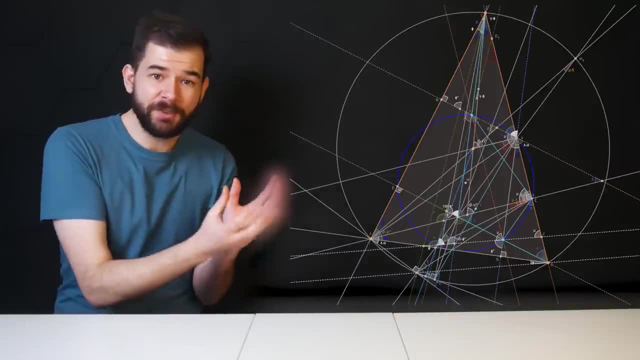 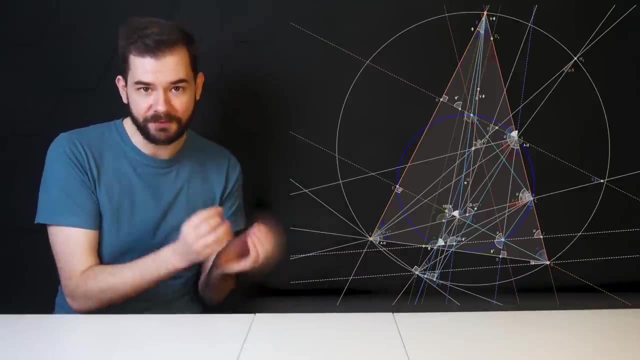 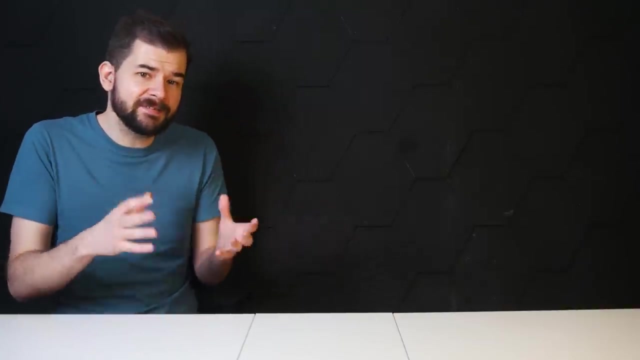 Does this matter? Yes, because we're in the land of plain geometry, which isn't some untapped wilderness of mathematical usefulness. It's a playground squarely in the domain of beauty. And what makes something beautiful? I don't know. It isn't the length of the proof, as shorter isn't always better, and it isn't simplicity. 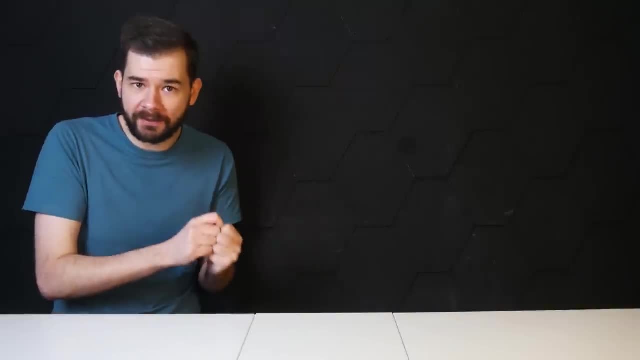 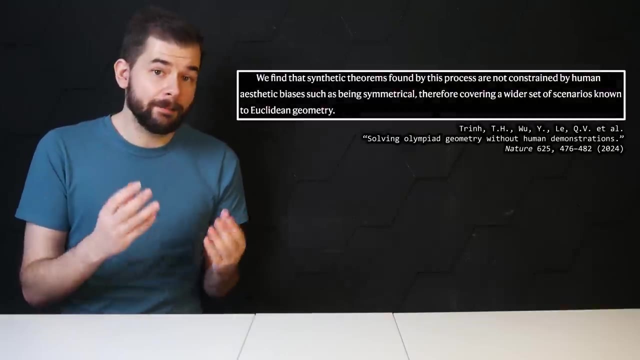 as too simple, often hides or disguises the inner workings. We just know it when we see it, and I don't think AI has come close to capturing beauty yet. There's a line about aesthetics in the Alpha Geometry paper: how alpha geometry might discover. 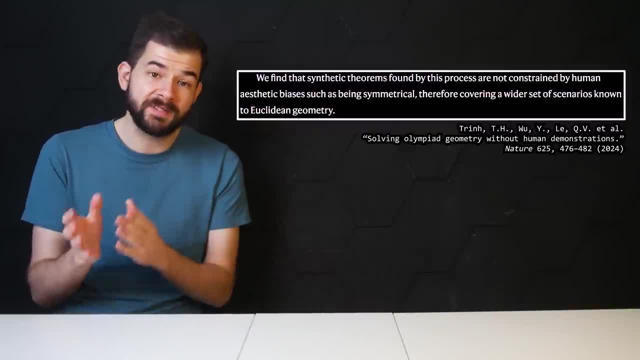 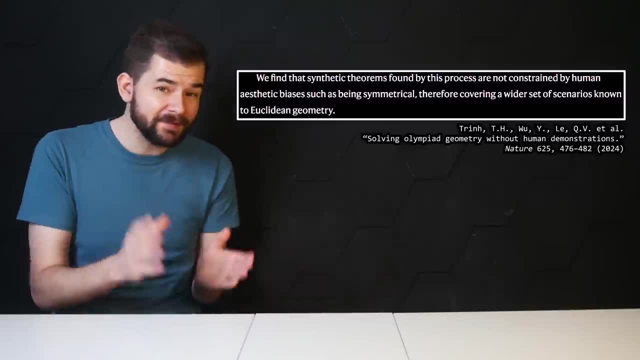 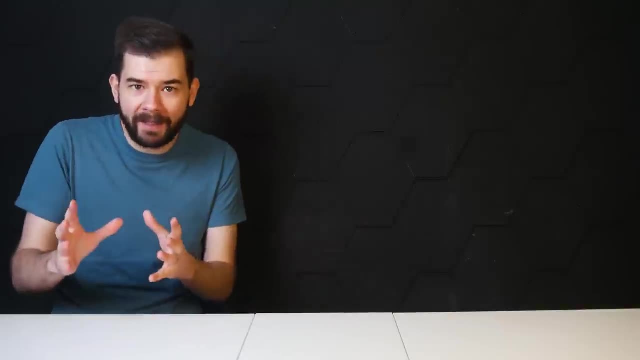 some plain geometry results, overlooked by us humans, because it isn't biased towards symmetry or that which is aesthetically pleasing And great. you do you alpha geometry. but if it isn't aesthetically pleasing, why do we care? Mathematics is often seen as something that's purely logical: it's black and white and 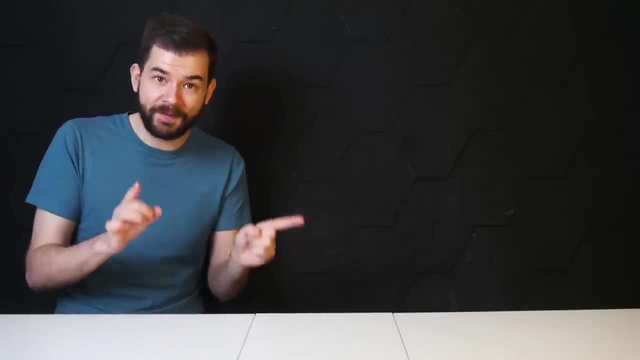 we love it for that, but we also love it for the aesthetics. Like, be honest, If I made a video saying here's an ugly geometry, what would you say? I'd be like, well, that's what I want. 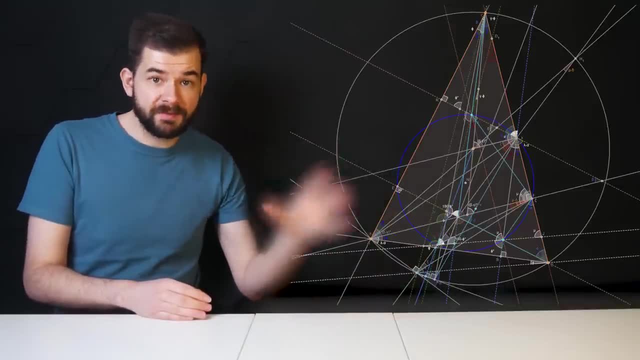 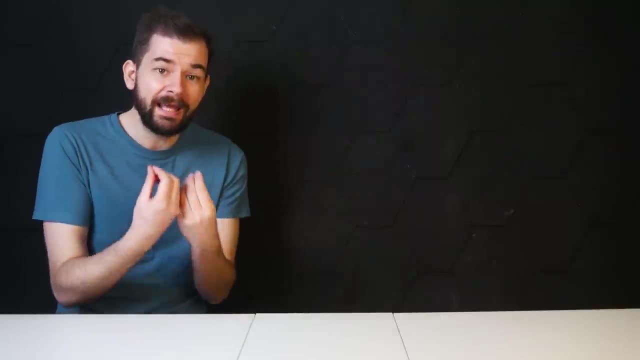 Here's an ugly geometrical result and here are the 100 difficult steps it takes to get there. Would you care about that? No, I curate topics that expose mathematical beauty, Even when the solution is kind of ugly. I try to make every step intuitive so we can. 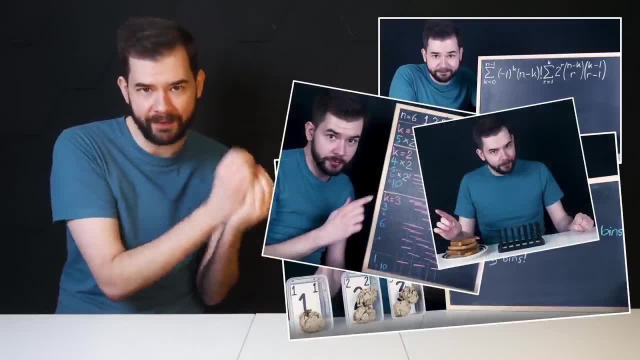 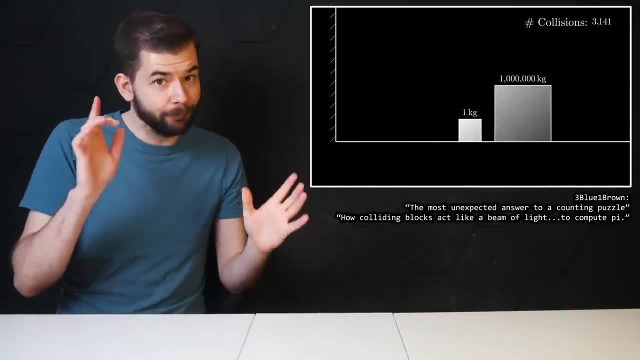 appreciate the symmetry, the hidden magic and the beauty within 3Blue1Brown's video on collisions printing pi. it's a jaw-dropping result, but we all watched the whole video Because the real awe comes not from the results. 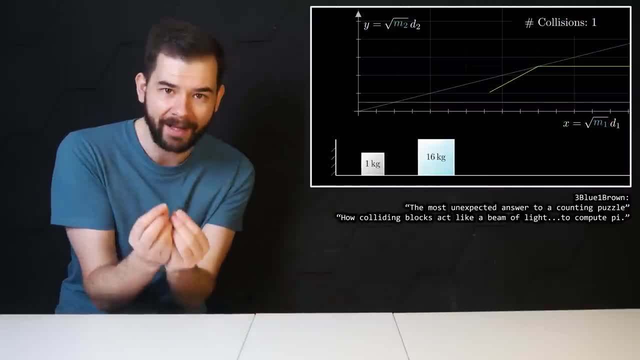 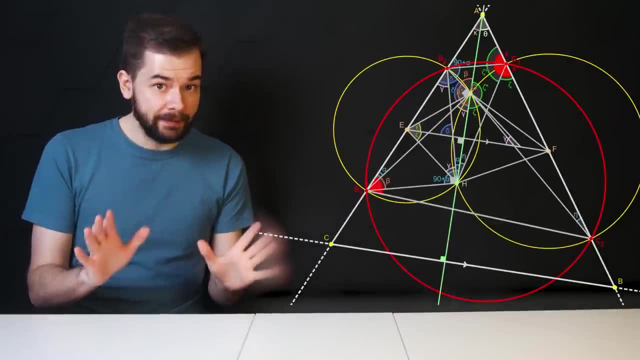 It's the results, Not from seeing the answer, but from seeing why. That's what we love, That's what inspires us, Not this. I want to be super clear here: I am not criticising Alpha Geometry or the authors of this paper.